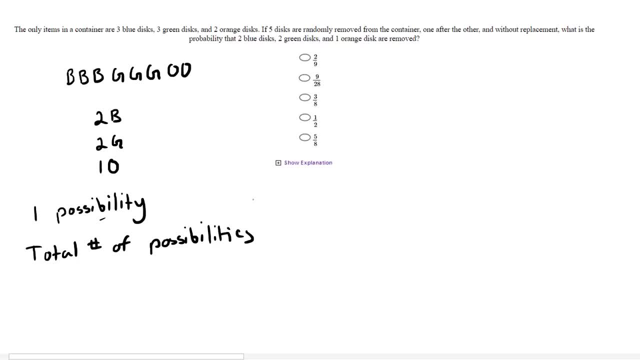 of one possibility, And this is the possibility I'm going to look for. Remember, I'm choosing five things: one, two, three, four, five. I just want it to be BB, GG and O. Now, keep in mind this is. 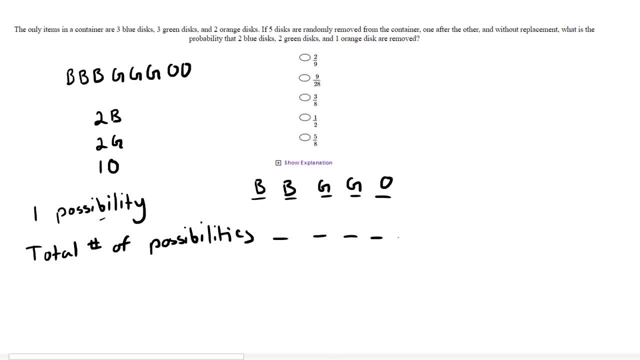 only one possibility, because I could also have, for example- I'll erase this, but I'll show you I could also have GB, BG and then O right. So I have more than one possibility here, But I'm only going to have one possibility here. So I'm going to have one possibility here, But I'm only going to. 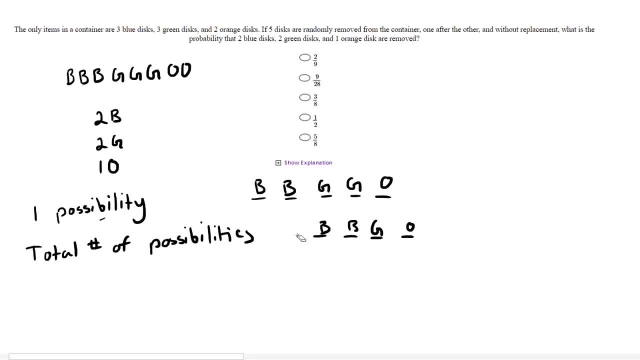 calculate the probability of one possibility, which shouldn't be too difficult. That's just a straight up independent probability problem. So what's the chance that I pull out a, B on my first go? Well, that would be three over eight, right, Do you agree? What's the chance that I pull out? 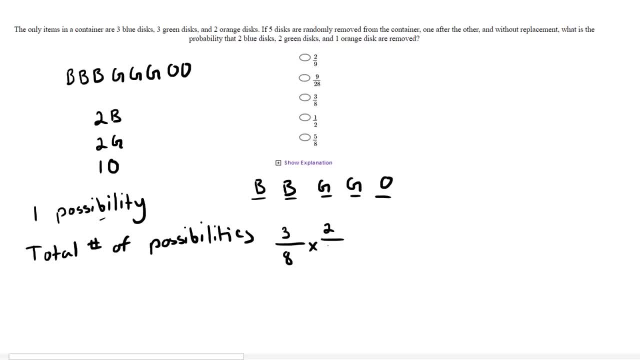 another B on my second go. That would be two over seven, And then the probability I get a G would be three over six. The probability I get another G would be three over seven, And then the probability I get another G would be two over five. And then, finally, how many O's do I have? I have two O's. 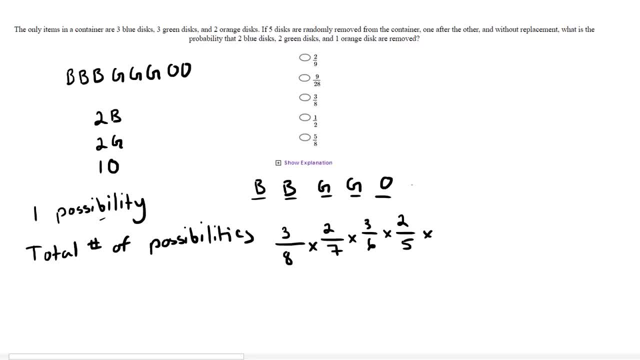 How many do I want? I want only one of them, but I do have two of them, So the chance of getting it would be two over four, like that. Now, before I try to do this math problem, I'm going to do some. 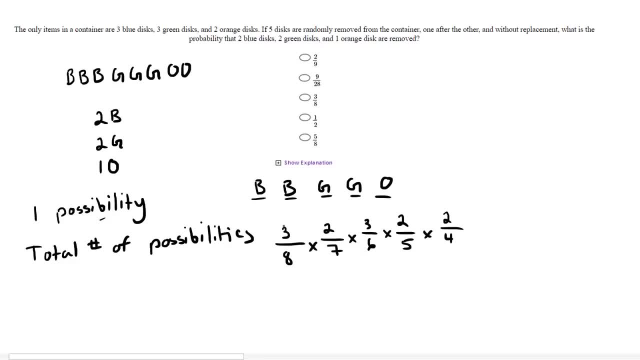 simplification. So do you see, three times two? Well, three times two equals six. right, So I can cross out the three and the two and also cross that out, right there? Do you see two times two? Well, two times two equals four. 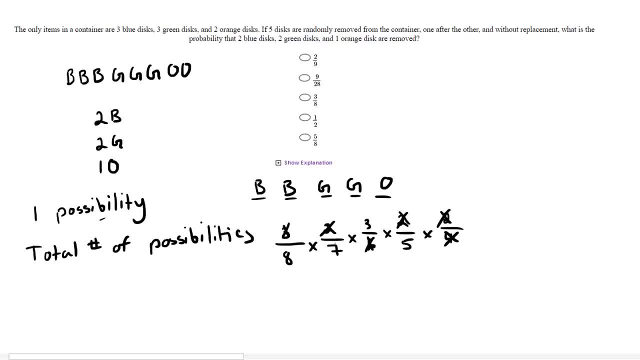 So I cross that out right there and see how much easier this math problem is. So now we have three on the top and we have 56 times five. What's that going to be? 280 on the bottom? So this is the probability of just one of these possibilities. So now the question is how many of these? 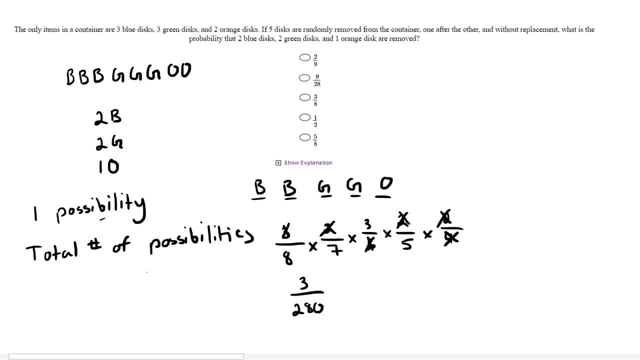 possibilities do I have? Okay, well, think about it as a five-letter word and the word is B-B-G-G-O. That's the word. How many ways can I arrange that? Right, And there's actually a formula that you can memorize. So take, for example, the word: 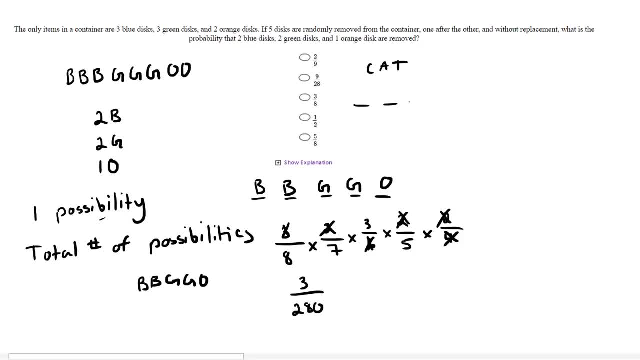 cat. So you have one, two, three. Well, if I want to rearrange this, how many different possibilities, how many choices do I have? I have three. I can have a C, an A or a T. So I say, okay, three. 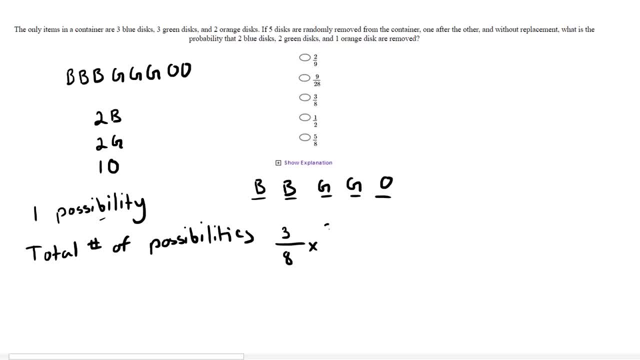 chance that I pull out another B on my second go. That would be two over seven, And then the probability I get a G would be three over six. The probability I get another G would be three over seven. So what's the probability that I pull out another G would be three over six. 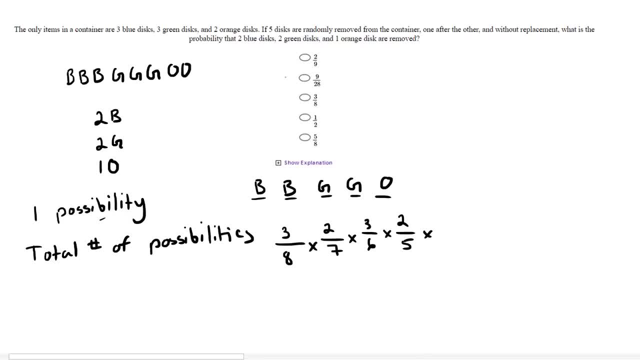 be 2 over 5.. And then, finally, how many O's do I have? I have two O's. How many do I want? I want only one of them, but I do have two of them. So the chance of getting it would be 2 over 4, like. 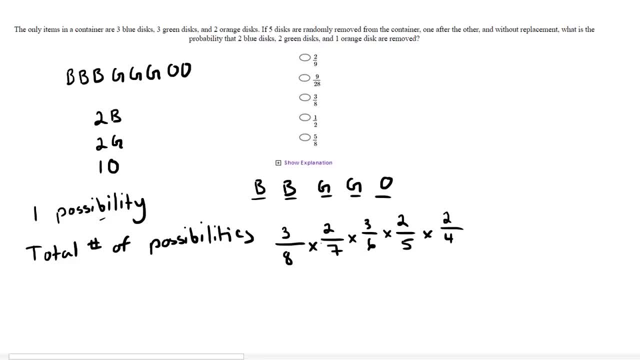 that Now, before I try to do this math problem, I'm going to do some simplification. So do you see 3 times 2? Well, 3 times 2 equals 6, right, So I can cross out the 3 and the 2 and also cross. 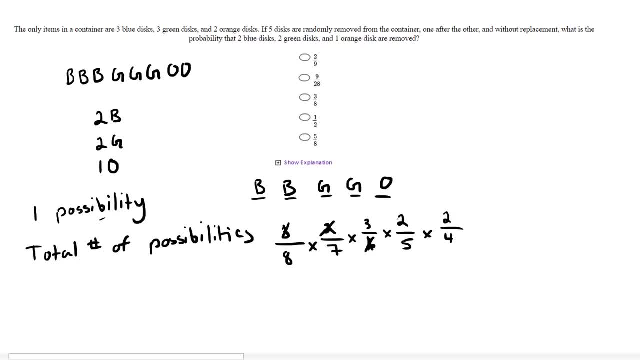 that out right there. Okay, do you see 2 times 2?? Well, 2 times 2 equals 4.. So I cross that out right there and see how much easier this math problem is. So now we have 3 on the top And we 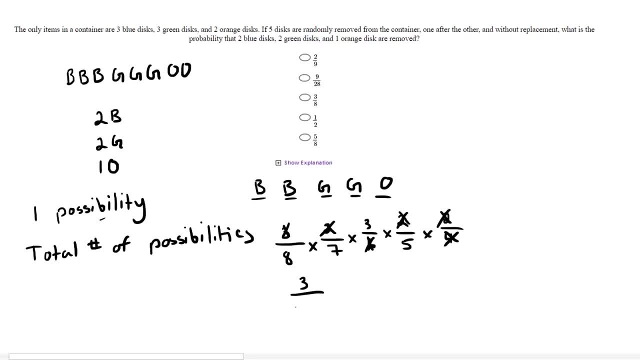 have 56 times 5.. What's that going to be? 280 on the bottom. So this is the probability of just one of these possibilities. So now the question is: how many of these possibilities do I have? Okay, well, think about it as a five letter word, And the word is: 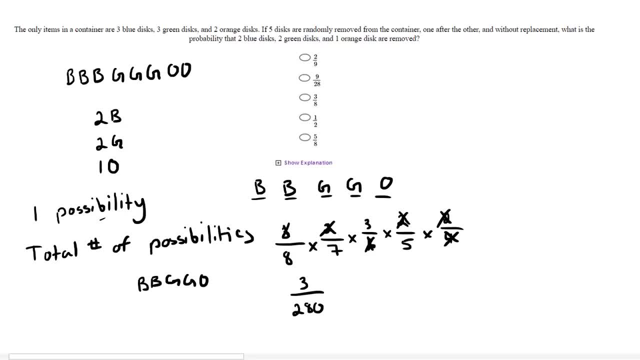 B, B, B, G, G, O, That's the word. How many ways can I arrange that right? And there's actually a formula that you can memorize. So take for example, the word cat, So you have 1,, 2,, 3.. Well, 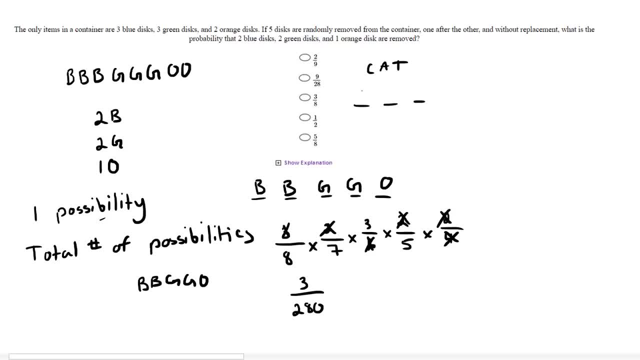 if I want to rearrange this, how many different possibilities, how many choices do I have? I have three. I could have a C, an A or a T. So I say, okay, three. how many choices? Two and then one. 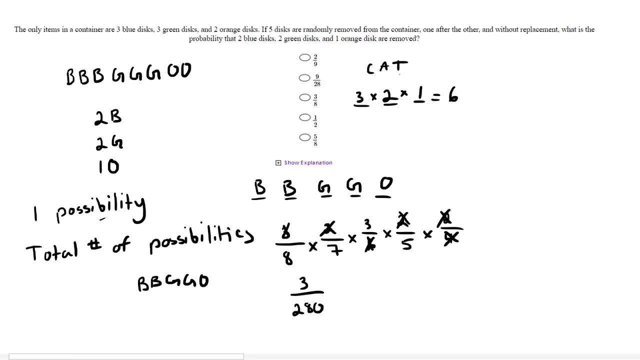 choice. Multiply all these together. You have six different ways to arrange that, But if you take a word like egg, for example, you also have three letters. The problem is you have a double G. So what that means is you can't just do three times, two times one, because that's not accurate. 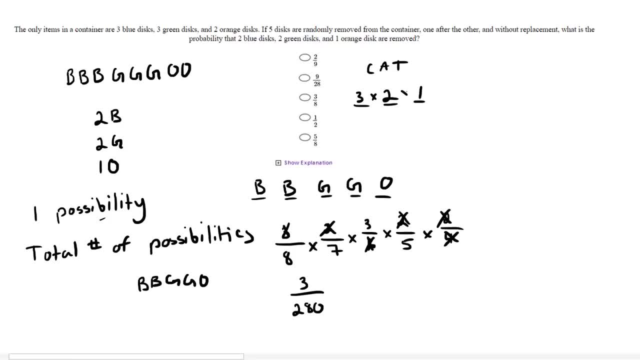 how many choices? Two and then one choice. Multiply all these together. You have six different ways to arrange that, But if you take a word like egg, for example, you also have three letters. The problem is you have a double G. 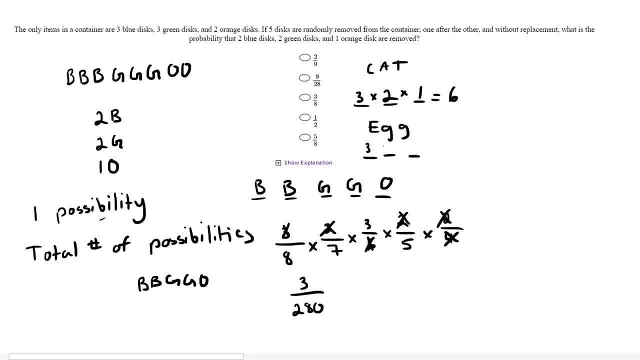 So what that means is you can't just do three times two times one, because that's not accurate with the double G. The double G kind of gets in the way, causes the number of possibilities to go down. So the formula is actually: you take the total number, like that, and then you just put on. 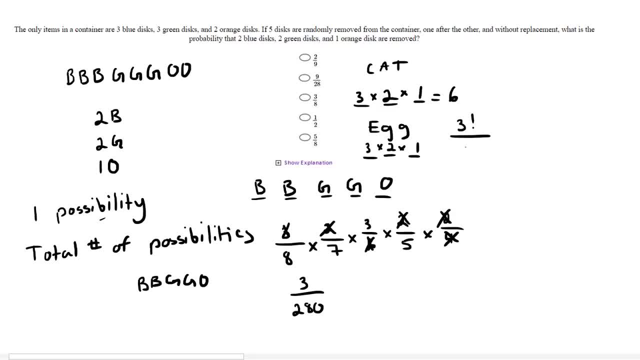 the bottom the number of repeats. So how many Gs do I have? I have two Gs like that. So really the total possibility is going to be just three. Same thing here, right, You have five on the top. how many Bs do I have? Two Bs? How many Gs do I have Two Gs, And this is going to equal five. 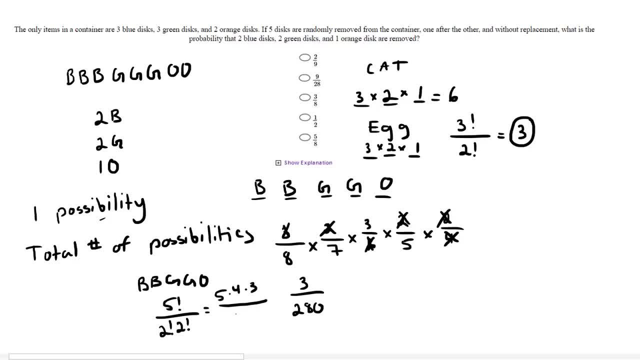 times four times three over two, like that. And then what are you going to get? You're going to get 20, 60. So this is going to equal 30.. All right, so now we are ready to solve the problem. 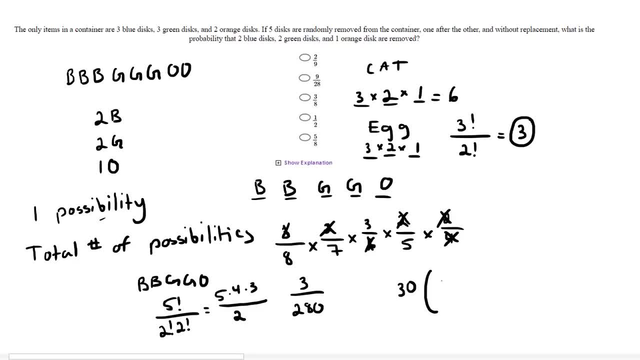 30. Remember, this is the total number of possibilities times the probability of one possibility over 280. And that's going to equal 30. So I'm going to get 20,, 60, and then I'm going to equal. well, we can simplify this a little bit. So if you cross out this zero and this zero, 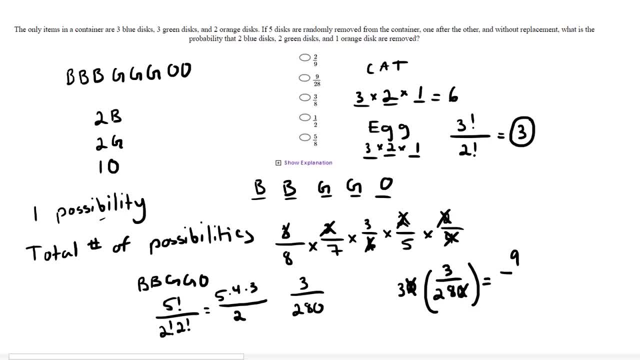 you're really getting three times three over 28.. You're getting nine over 28 right there. So it looks like the correct answer is going to be B. Now again, let me reiterate my process. here I found the possibility or the probability of only one of these cases, And the case I found 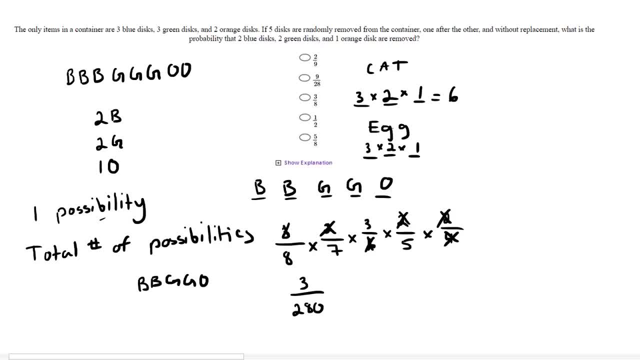 with the double G. The double G kind of gets in the way, causes the number of possibilities to go down. So the formula is actually: you take the total number, like that, and then you just put on the bottom the number of repeats. So how many Gs do I have? I have two Gs like that. So really the 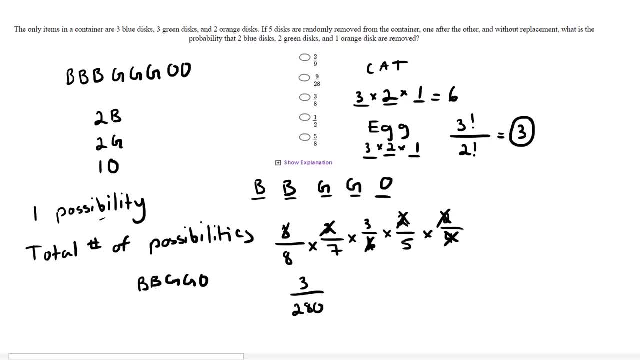 total possibilities are like that: So I have two Gs, So I have two Gs, So I have two Gs, So I have three. So the total number of possibilities is going to be just three. Same thing here, right You? 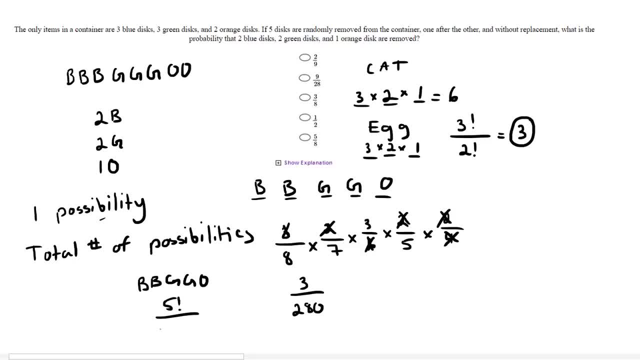 have five on the top. How many Bs do I have Two Bs? How many Gs do I have Two Gs? And this is going to equal five times four times three over two, like that. And then what are you going to get? 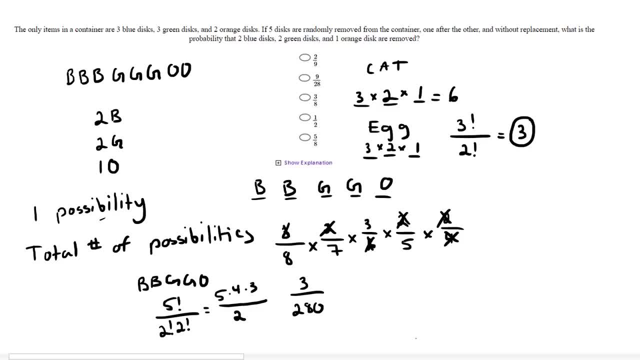 You're going to get 20, 60. So this is going to equal 30.. All right, so now we are ready to solve the problem. 30. Remember, this is the total number of possibilities Times the probability of one possibility over 280. And that's going to equal. well, we can. 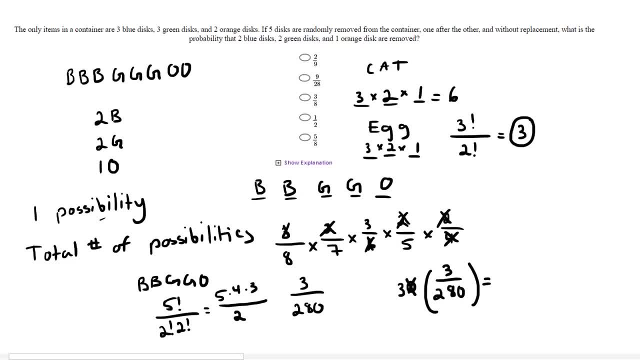 simplify this a little bit. So if you cross out this zero and this zero, you're really getting three times three over 28.. You're getting nine over 28 right there. So it looks like the correct answer is going to be B. Now again, let me reiterate my process. here. I found the possibility. 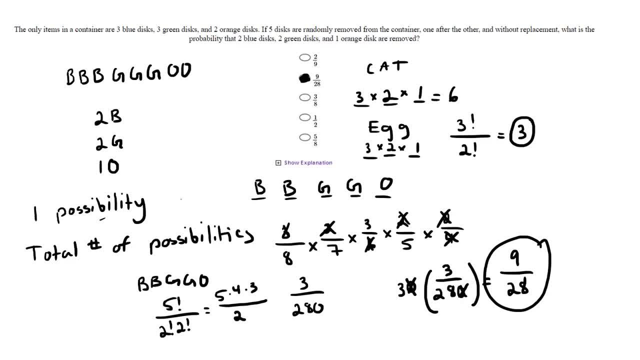 or the probability of only one of the two possibilities. So I'm going to get three times three over the total number, and then we're going to get the other two possibilities over the same number. So you're going to get three times the probability of one of the two possibilities. 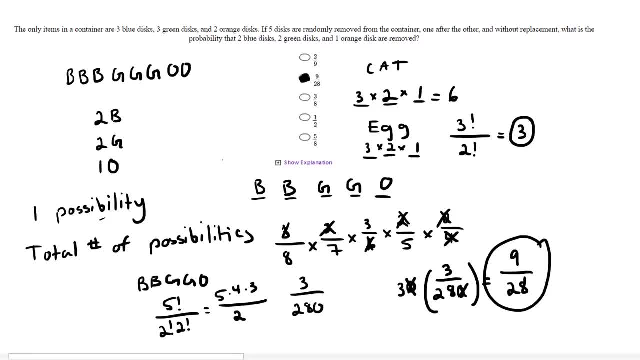 But that's obviously not the only case, because I could also have B, G, G, O, B, right. So now the next thing I did is: how many of these different cases do I actually have? And that's where the kind of this formula came into play, where you have the total number of like letters or whatever. 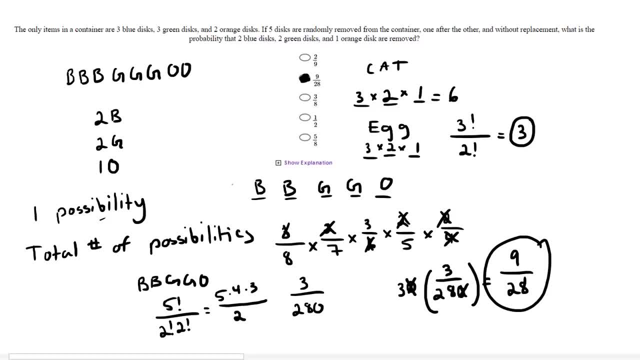 was BBGGO, But that's obviously not the only case, because I could also have BGGOB, right. So now the next thing I did is: how many of these different cases do I actually have? And that's where the kind of this formula came into play, where you have the total. 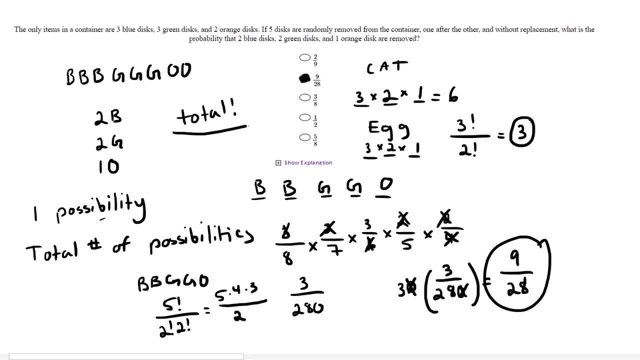 number of like letters, or whatever you want to call it, over the repeats, over the repeat like that. Okay, so final answer is nine over 28.. This is a pretty tough problem. The chance you see this on the GRE is probably pretty low. 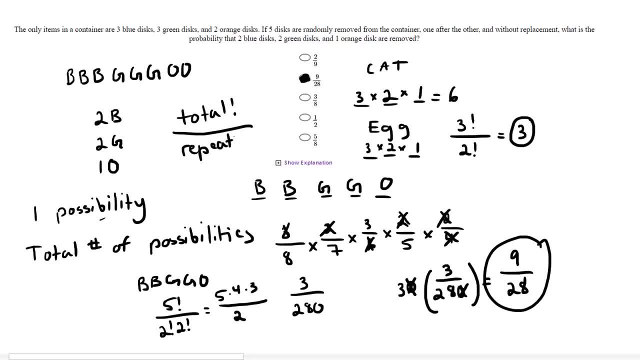 you want to call it over the repeats, over the repeat, like that. Okay, So final answer is nine October 28.. This is a pretty tough problem. The chance you see this on the GRE is probably pretty low, And if you do, you'd only see one of these bad boys For most people. I would suggest you. 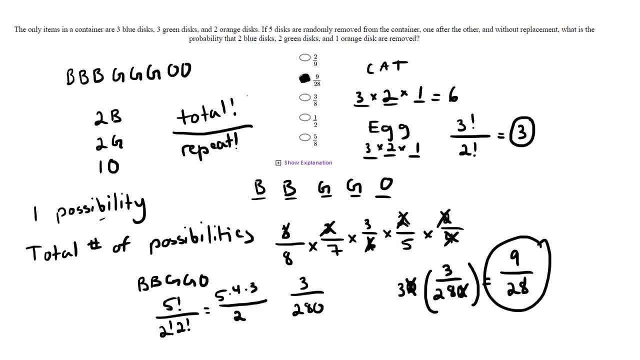 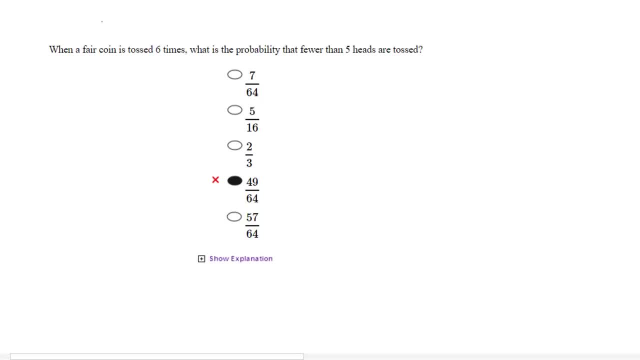 skip it, Unless you're trying to get like a 170 or something like that. But anyway, that's how I would solve it. Okay, so here's the second one that the Reddit user requested, And it says: when a fair coin is tossed six times, what is the probability that fewer than five heads are tossed? 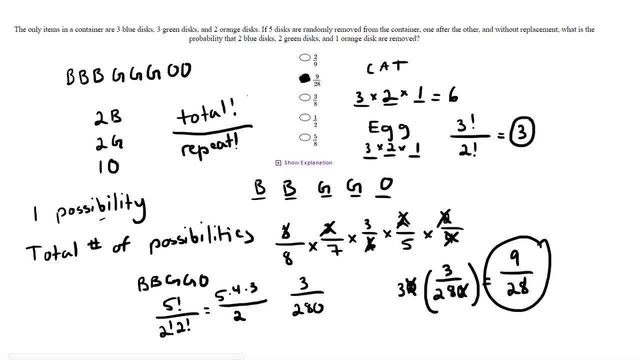 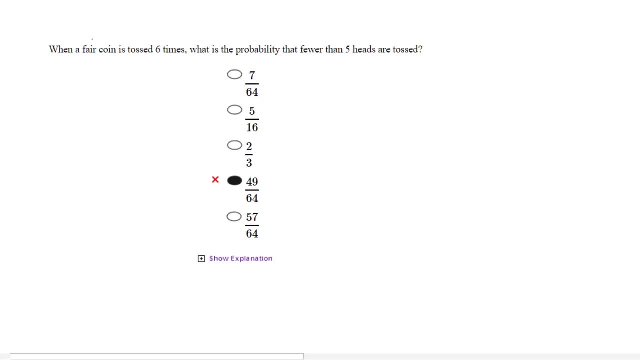 do, you would only see one of these bad boys for most people. i would suggest you skip it, um, unless you're trying to get like a 170 or something like that. but anyway, that's how i would solve it, okay. so here's the second one that the reddit user requested, and it says: when a fair 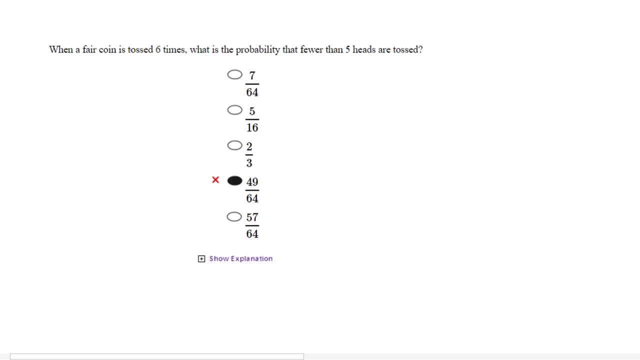 coin is tossed six times, what is the probability that fewer than five heads are tossed? let's just do this one right here. when you toss a coin six times, how many possibilities are there? well, you can only get a heads and a tails right. so in my first toss i have two choices. it can either be: 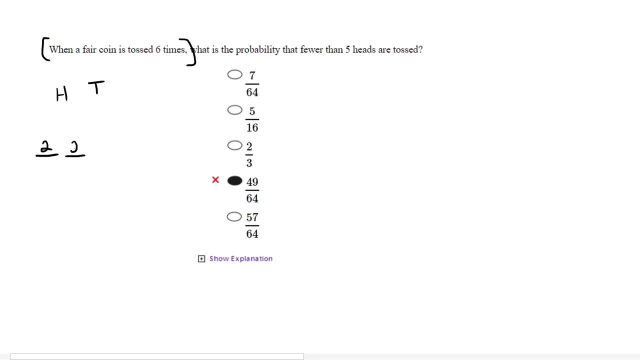 heads, or it can be tails in my second choice. i have two in my third choice, or in my third flip two, in my fourth flip two and my fifth flip two, and then in my sixth flip two. so what the? the total number of possibilities are two. and then in my fourth flip two and then in my sixth flip two. 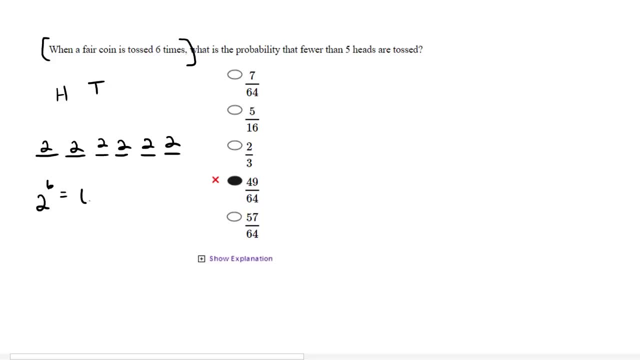 is actually two to the six, which equals 64.. so we're looking at 64 total possibilities here. 64 total possibilities- okay, does that make sense? so one thing i could do is i could immediately eliminate this one, because 6 plus 4 equals 10 and it's not a multiple of three. so this is definitely 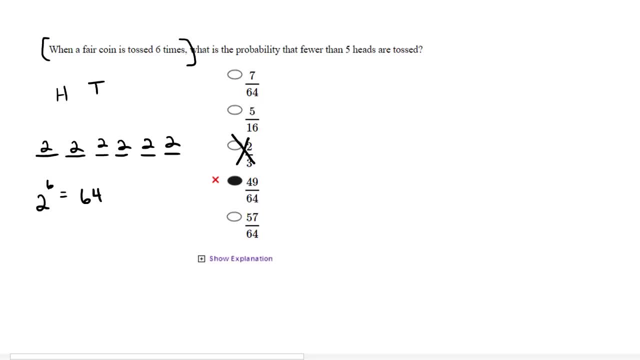 wrong right there. but 16 is a factor of 64.. 64 is obviously a factor of 64, 64, yeah, so we can just immediately eliminate C. that's just wrong. Okay, now we go to the second part. What is the probability that fewer than five heads are tossed? 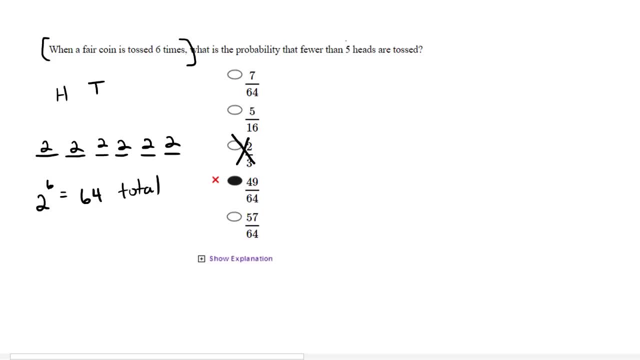 So remember, we have 64 total possibilities. So what would make me happy Fewer than five heads? well, zero heads would make me happy. One head, two head, three head and four head, that would make me happy. What would make me unhappy? It would be five heads or six heads. 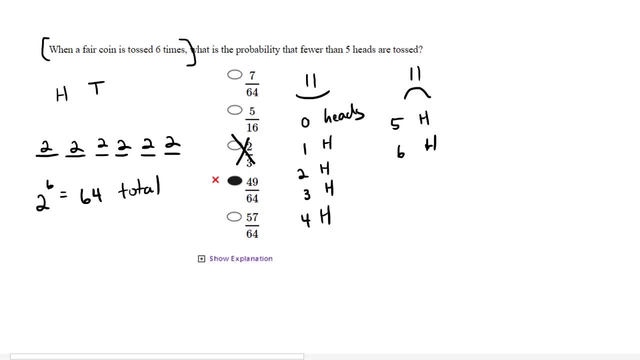 Now notice: if you had to calculate these individually, you would have to do four or five, five different calculations. with happy one, two, three, four, five. But with unhappy you only have to do two calculations. So the better approach here is calculate the things. 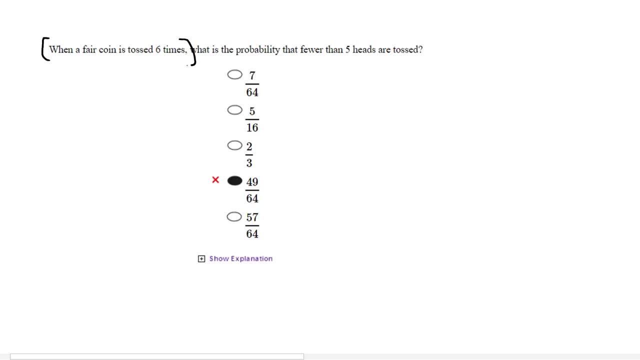 Let's just do this one right here. When you toss a coin six times, how many possibilities are there? Well, you can only get a heads and a tails right. So in my first toss I have two choices: It can either be heads or it can be tails. In my second choice I have two. In my third choice, or in my 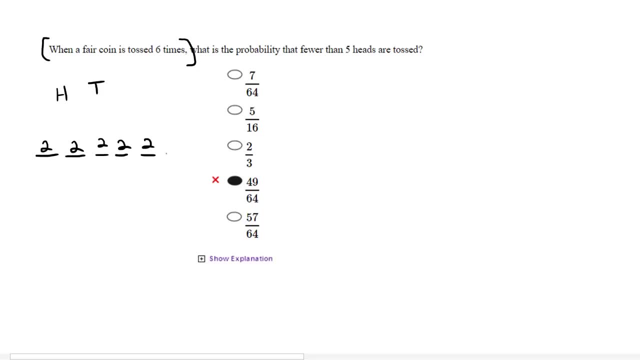 third flip two, and my fourth flip two, and my fifth flip two, and then in my sixth, flip two. so what? the? the total number of possibilities is actually two to the six, which equals 64. so we're looking at 64 total possibilities here. 64 total possibilities, okay. does that make sense? so one thing i could: 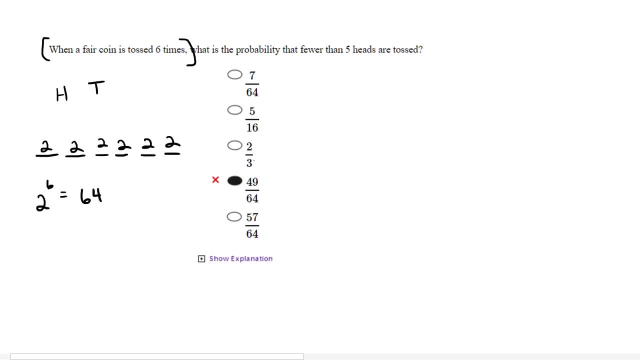 do is i could immediately eliminate this one, because 6 plus 4 equals 10 and it's not a multiple of three. so this is definitely wrong, right there. but 16 is a factor of 64. 64 is obviously a factor of 64, 64. yeah, so we can just immediately eliminate c. that's just wrong. okay, now we go to the second. 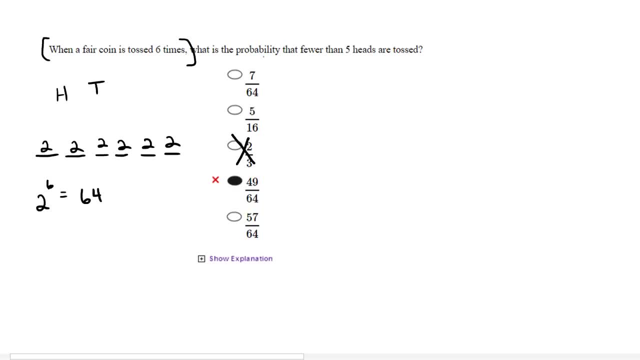 part. what is the probability that fewer than five heads are tossed? so remember, we have 64 total possibilities. so what would make me happy fewer than five heads? well, zero heads would make me happy. one head, two head, three head and four head, that would make me happy. 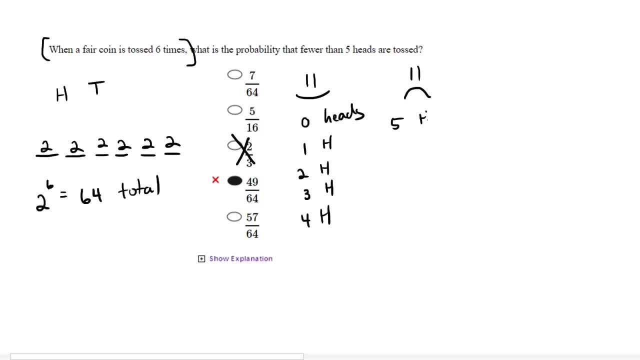 what would make me unhappy it would be five heads or six heads. now notice: if you had to calculate these individually, have to do four or five different calculations. with happy One, two, three, four, five. But with unhappy you only have to do two calculations. So the better approach here is calculate the things. 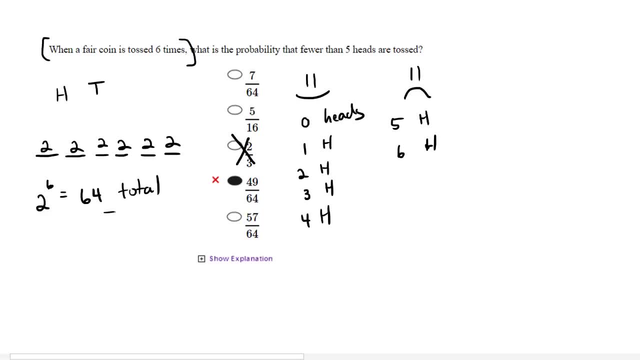 that make me unhappy and subtract it from the total, And that will give you what makes you happy. It's a much faster approach. So let's calculate the probability of getting this right here. All heads, six heads, because that's the easier one. So the probability of getting six: 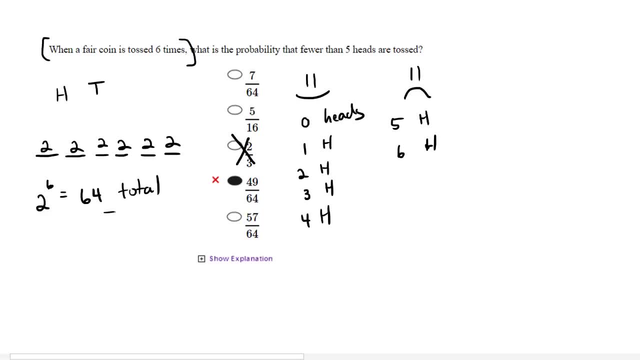 that make me unhappy and subtract it from the total, and that will give you what makes you happy. It's a much faster approach. So let's calculate the probability of getting this right here. all heads, six heads, because that's the easier one. So the probability of getting six: 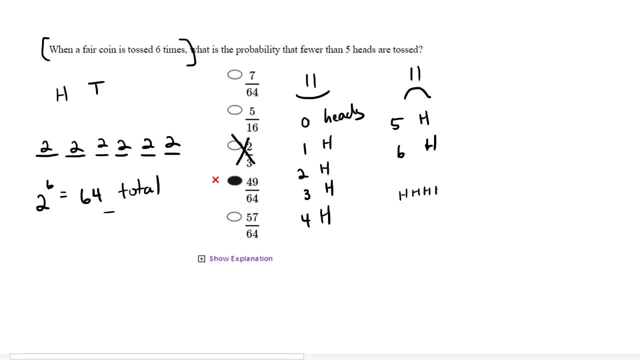 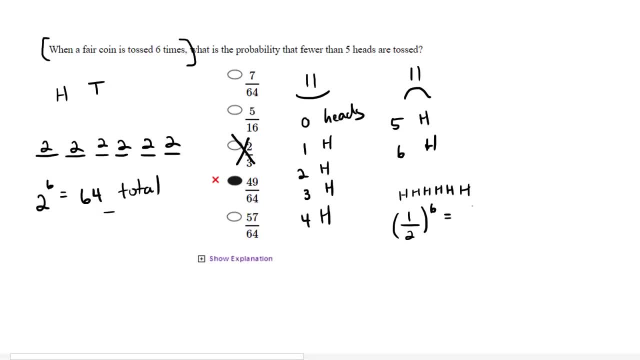 one half to the sixth right, And that's going to equal one over 64.. So there's only one possibility. This only happens one time out of 64.. So let's go ahead and subtract out the one. All right, So the one is subtracting out, and now our new number is 63. 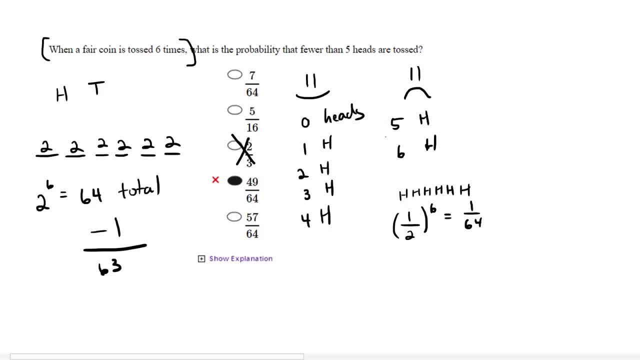 So the next question is: five heads, Just like in that previous problem: calculate the probability of this happening one time. Okay, so let's calculate the probability of h, h, h, h, h, tails. Well, the first five h's are going to be one half to the fifth power, And then getting the tails is 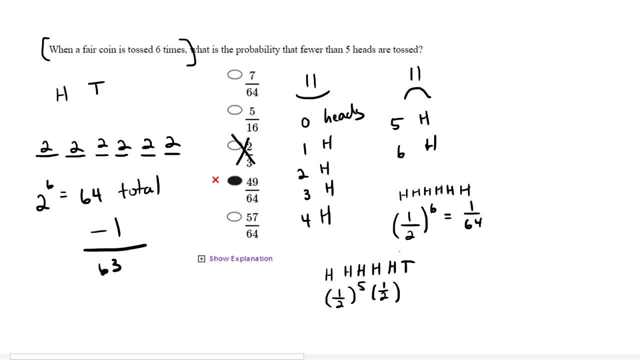 also going to be just one half, But here's the difference, right? So this looks like it equals one over 64, right? But here's the difference. This tails can move, So this tails can go here. okay, That's another case. It can go here. That's another case. Here, here or here. So how many? 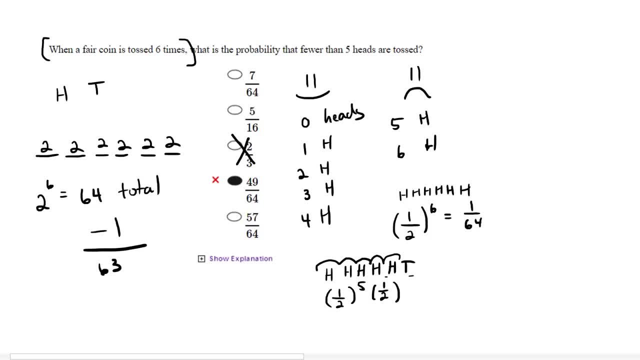 total cases is that? Well, that's going to be one, two, three, four, five, six, So six total cases. So I need to multiply this by six, right? So what I'm getting is actually one over 64, same thing. 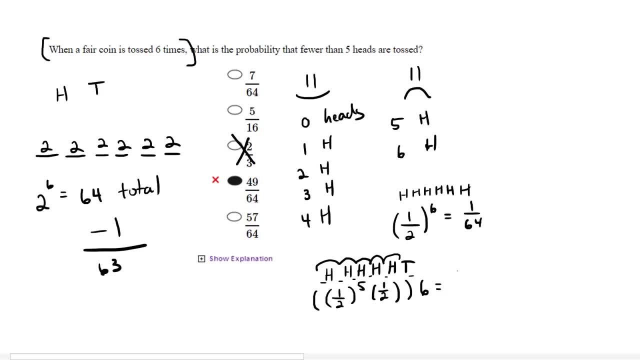 here times six, because that tail can move to six different places. So there's actually six over 64 possibilities here. So of the 64, six of them have this kind of tails somewhere, either at the end, the front or in between the h's. So, finally, what do I need to do? Subtract this out, Remember. 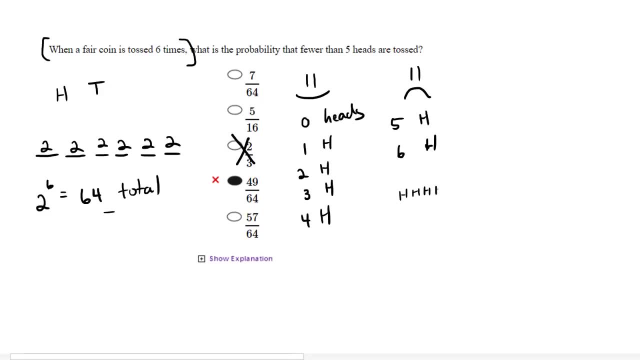 heads would be head, head, head, head, head and then finally head. Well, that's just going to be one half to the six right And that's going to equal one over 64. So there's only one possibility. 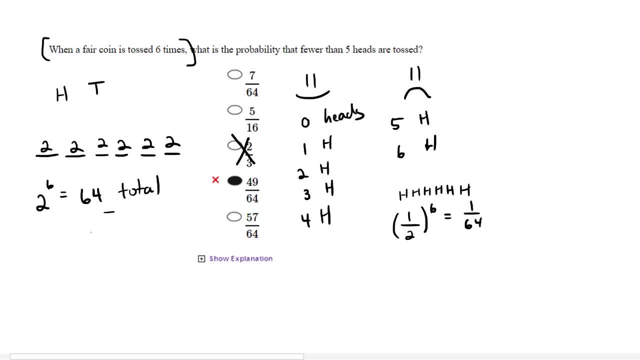 There's only. this only happens one time out of 64. So let's go ahead and subtract out the one. All right, So the one is subtracting out, and now our new number is 63.. So the next question is: five heads, Just like in that previous problem: calculate the probability? 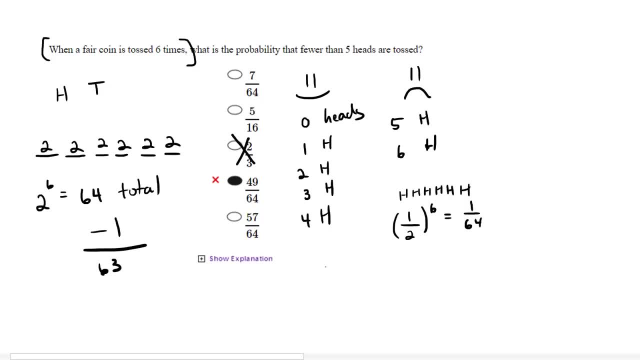 of this happening one time. Okay, so let's calculate the probability of H, H, H, H, H, tails. Well, the first five H's are going to be one half to the fifth power, And then getting the tails is a half to the fifth power, So that's going to equal one over 64.. So let's go ahead and 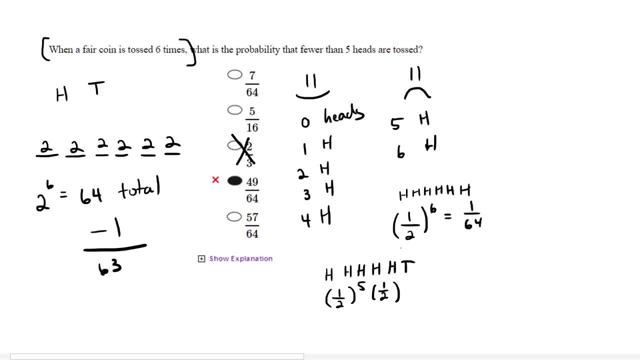 calculate the probability of H, H, H, H, H tails. Well, the first five H's are going to equal one half to the fifth power, And then getting the tails is also going to be just one half. But here's the. 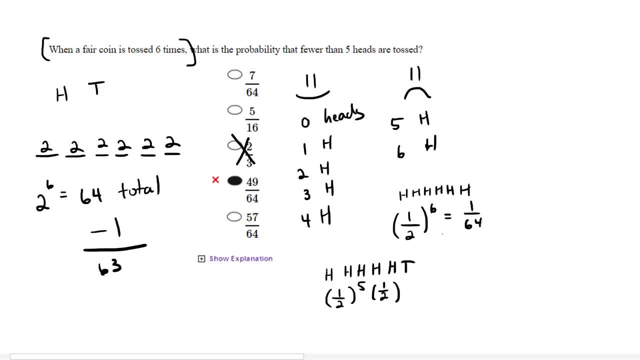 difference, right? So this looks like it equals one over 64, right? But here's the difference. This tails can move, So this tails can go here. Okay, that's another case it can go here. that's another case here, here or here. So how many total cases is that? Well, that's going to be 123456.. So six. 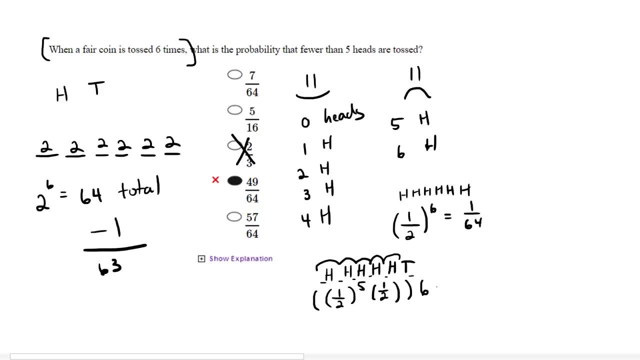 total cases. So I need to multiply this by six, Right? So what I'm getting is actually one over 64, same thing here times six, because that tail can move to six different places. So there's actually six over 64 possibilities here. So of. 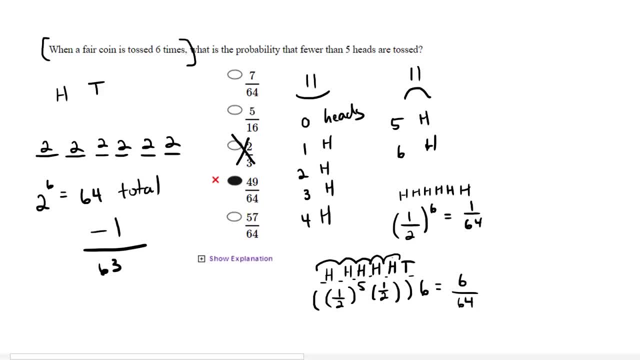 the 64,, six of them have this kind of tails somewhere, either at the end, the front, or in between the H's. So, finally, what do I need to do? subtract this out, Remember, because it makes me unhappy. So minus six, And then, finally, what do you get? 57.. 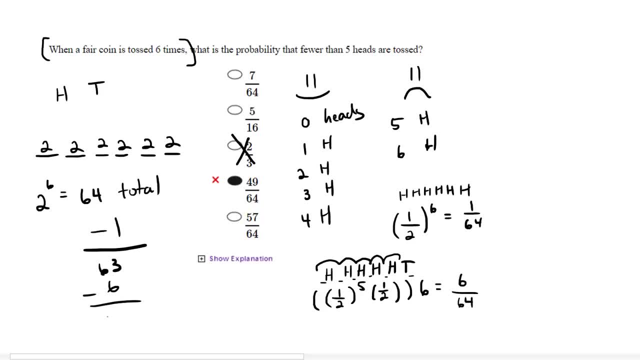 because it makes me unhappy. So minus six, And then, finally, what do you get? 57.. So 57 cases make me happy, because I subtracted out all of the unhappy ones And the total number of cases is 64.. 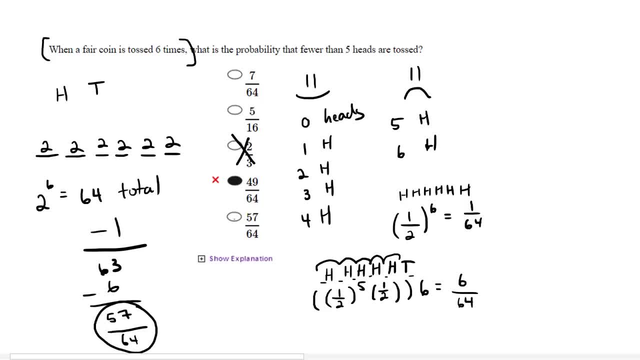 So the final answer is going to be 57 over 64.. Right there. Now what principle can we learn here? The main principle is that you can solve it the other way, the happy way. It's just you have to do five calculations By taking out the things. 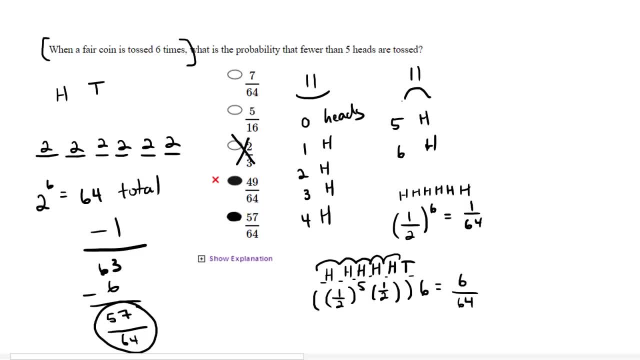 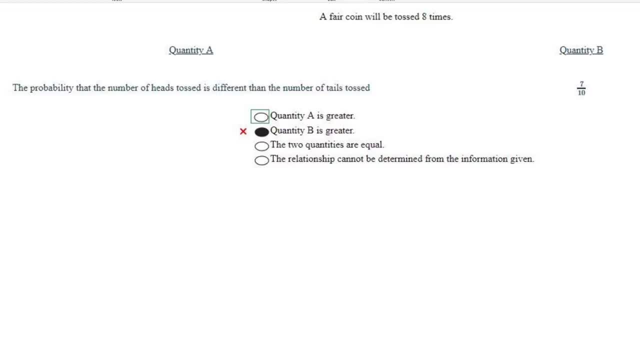 that make you unhappy. it's a much faster approach. All right, so for this next one. at the top it says a fair coin is tossed eight times, And from the previous one you know how to calculate the total number of possibilities. Just as a reminder, for each toss I have two. 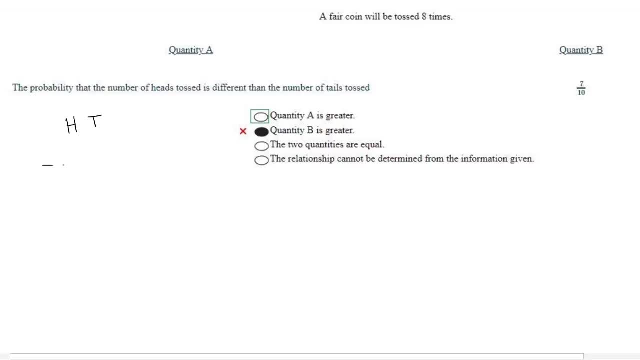 possibilities, heads or tails, right. So if you put eight of these- 12345678, and then you have a: two possibilities, two possibilities, two, two, two, two, two, two, and what you end up with is two to the eighth. Okay, And what does that equal? Well, two to the sixth. 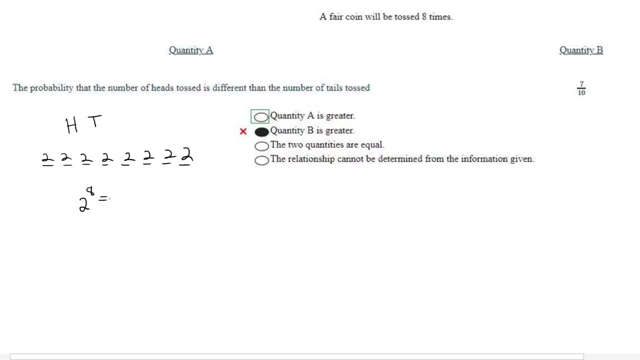 is 64. And then two to the seventh would be 128. And then this. so this is going to be 256 total possibilities. Alright, so what do I want? What will make me happy And what will make me unhappy? 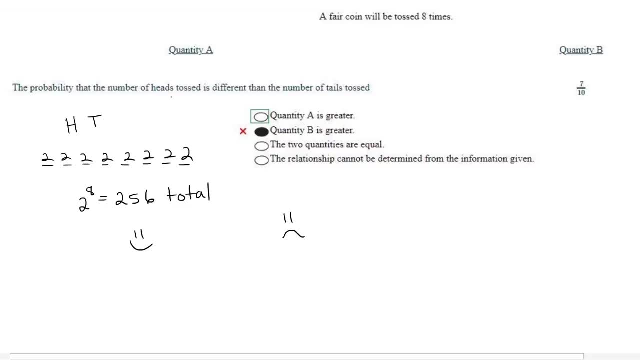 So the probability that the number of heads tossed is different than the number of tails tossed. So what makes me happy is just when the heads and tails are different. So heads- heads doesn't equal tails. So, just as an example, like heads, heads, heads, heads, heads. 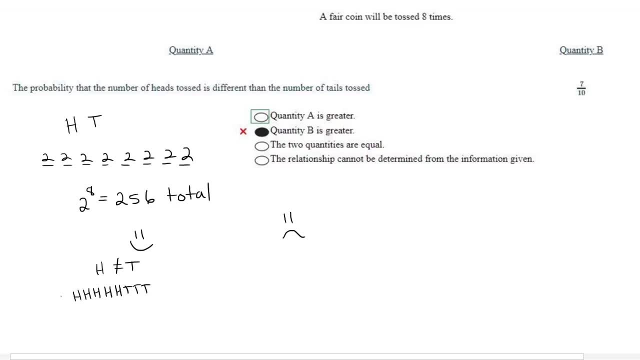 and then tails, tails, tails. this will make me happy, because there's five heads and three tails. what will make me unhappy? Well, the only thing that will make me unhappy is when I have an equal number heads, heads, heads, tails, tails, tails. So this makes me unhappy. What would be easier to? 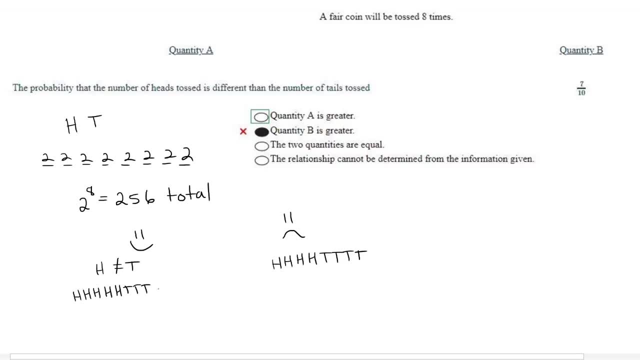 calculate with the happy cases or the unhappy cases. Well, let's say I have an equal number and I'm unhappy. Well, the happy cases, there's a lot of them, you know: one head, seven tails. seven heads, one tail. it's very time consuming. But in the unhappy case there's only one. 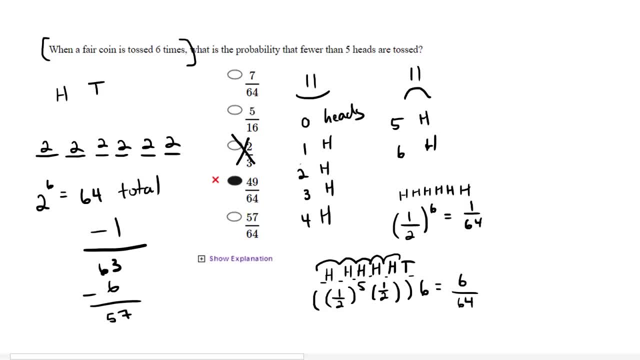 So 57 cases make me happy, because I subtracted out all of the unhappy ones And the total number of cases is 64. So the final answer is going to be 57 over 64, right there. Now what principle can we learn here? The main principle is that you can solve it the other way. 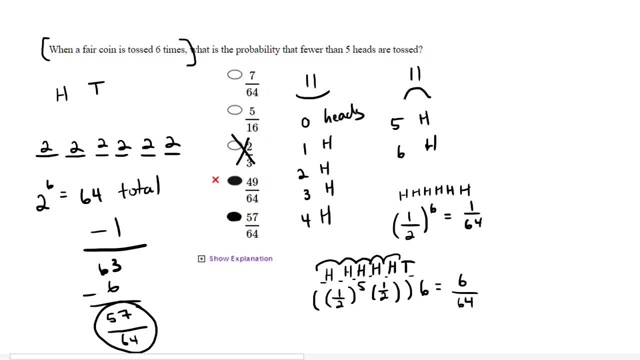 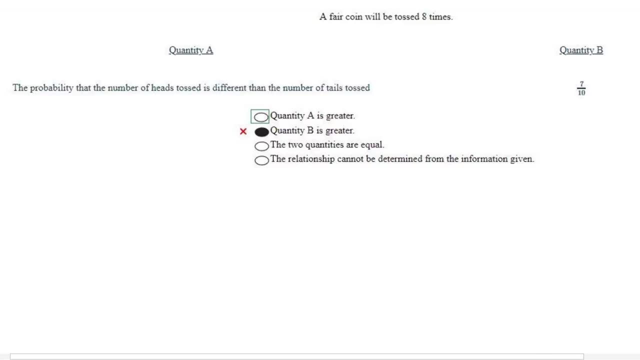 the happy way. it's just you have to do five calculations By taking out the things that make you happy and then yourself. it's a much faster approach. All right, so for this next one. at the top it says: a fair coin is tossed eight times And from. 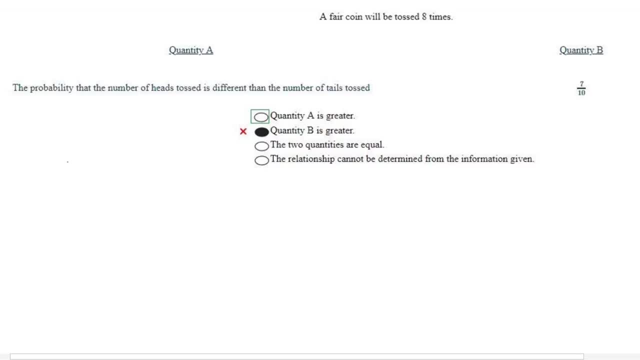 the previous one, you know how to calculate the total number of possibilities. Just as a reminder, for each toss I have two possibilities, heads or tails, right. So if you put eight of these, 123456,, six, seven, eight, And then you have a, two possibilities, two possibilities, two, two. 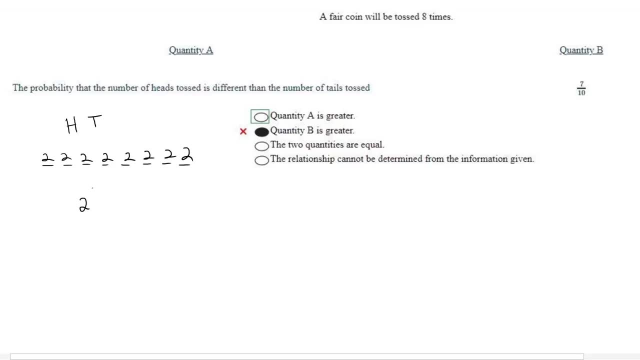 two, two, two, two, And what you end up with is two to the eighth. Okay, And what does that equal? Well, two to the sixth is a 64, and then two to the seventh would be one 28.. And then this: 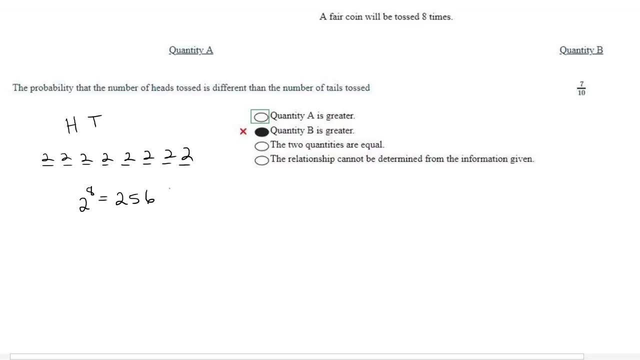 so this is going to be 256 total possibilities. All right, So what do I want? What will make me happy and what will make me unhappy? So the probability that the number of heads tossed is different than the number of tails tossed. So what makes me happy is just when the heads 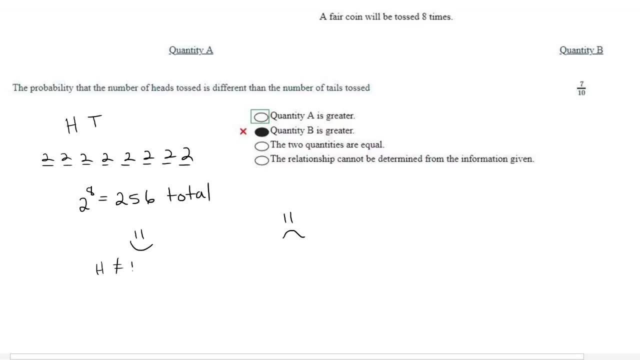 and tails are different. Heads doesn't equal tails. So, just as an example, like heads, heads, heads, heads, heads and then tails, tails, tails. This will make me happy, because there's five heads and three tails. What will make me unhappy? 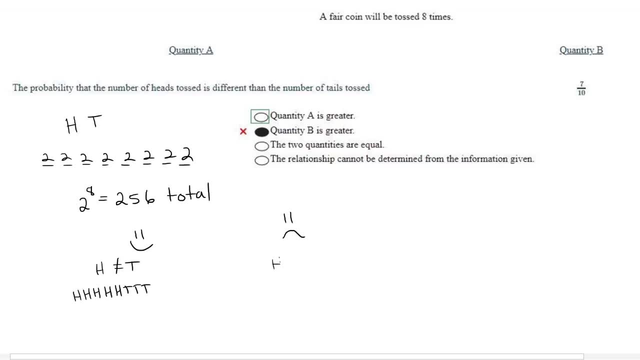 Well, the only thing that'll make me unhappy is when I have an equal number heads: heads, heads, tails, tails, tails. So this makes me unhappy. What would be easier to calculate with the happy cases or the unhappy? Well, the happy cases there's a lot of them, you know, one heads. 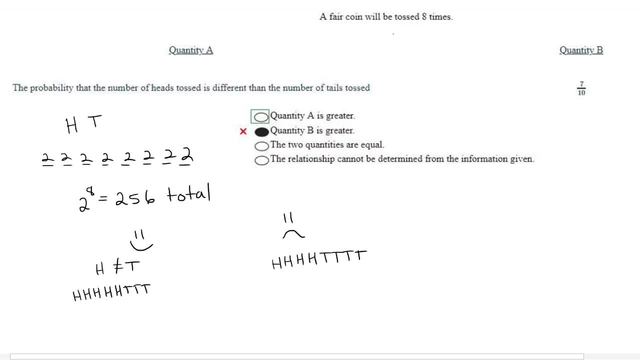 seven tails, seven heads, one tail. It's very time consuming, but in the unhappy case there's only one. there's only one case here that makes me unhappy. So it would be much easier to calculate the probability of this happening and then calculate the total number of. 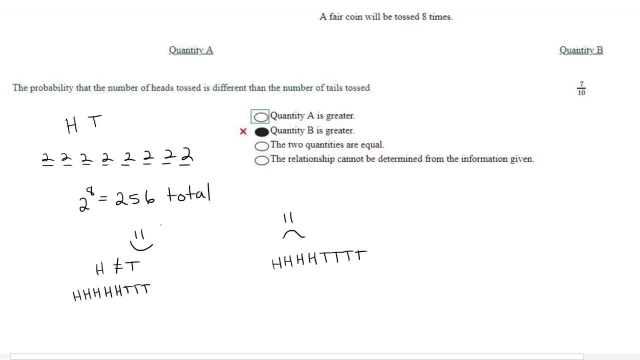 possibilities: Okay. So the total number of possibilities: 256,. what is the probability that this happens right here? Well, if I get four heads in a row, that's going to be one half to the fourth, Okay. And if I get four tails in a row, that's going to be one half. 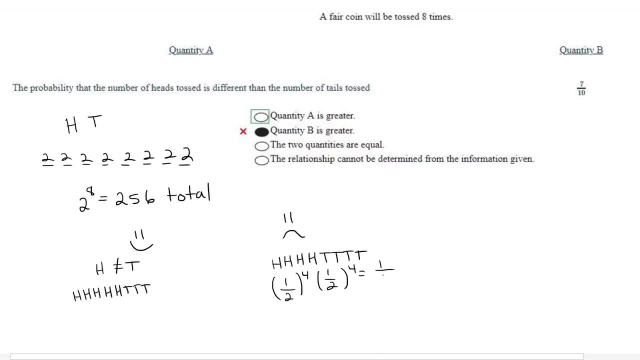 to the fourth, And that's going to equal one half to the eighth, just like before, And that's going to equal one over 256.. So this is just one case of the 256 right there. So the question is now, how many of these different cases? 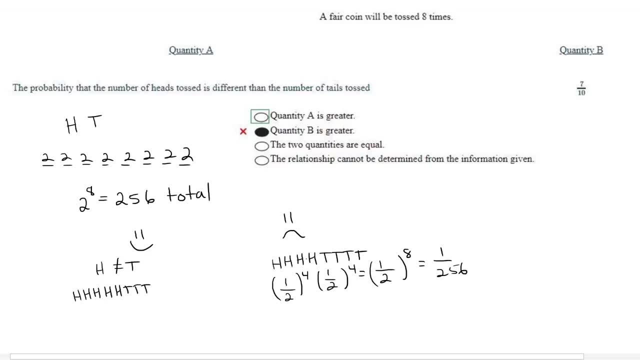 do I have where I have four H's and four T's. Remember, these T's can be in the middle of the H's or the H's can be in the middle of the T's, right? So we're just going back to our good friend. 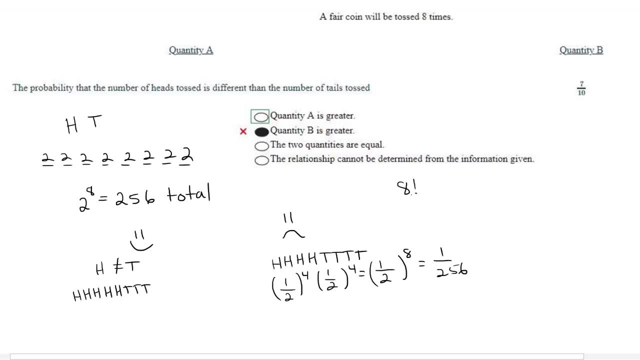 you know the total over the repeats. So the total is eight factorial. How many H's are there Four? How many T's are there Four? And so what do we get? We get eight times seven times six times five over four times three times two times one, And we can do a lot of. 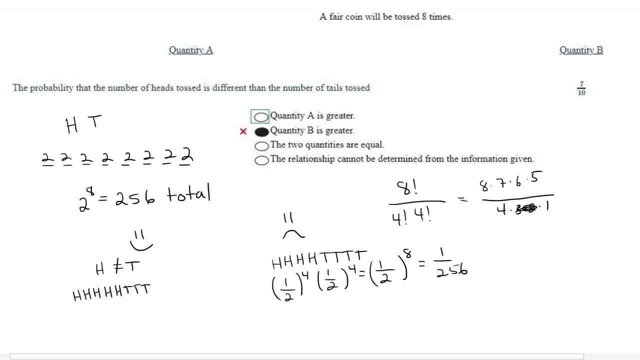 simplification here, right? So you know the three and the two. well, those go away, So does the six. that four goes away and that turns into a two. So what do we get? We get 35.. What's that? 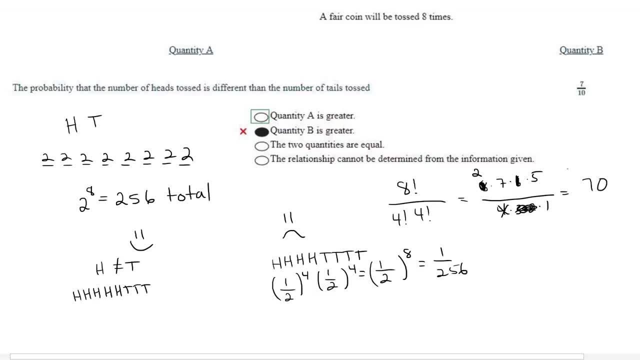 70.. All right, So we have 70 total possibilities. Now, remember, these possibilities make me unhappy, So I need to subtract them from two 56, two 56 minus 70. And what is that going to equal? That's going to equal, what is it? One 86.. Is that right? All right. So these number of 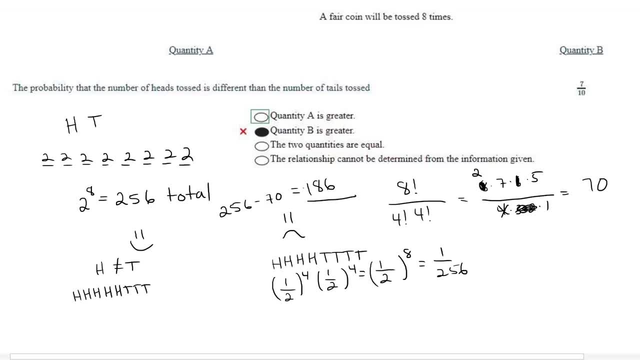 pot. these possibilities make me happy, because that means they're not equal, because I subtracted all the things that make me unhappy. So one, 86 over the total number, which is going to be two, 56. And then, finally, I'm going to compare this number to seven over 10 and see which one is. 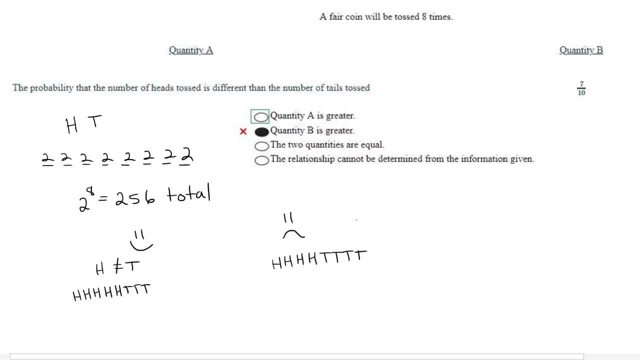 there's only one case here that makes me unhappy. So it would be much easier to calculate the probability of this happening and then calculate the total number of possibilities. Okay, so the total number of possibilities: 256.. What is the probability this happens right here? Well, if I get four heads in a row, that's going to be one half to the. 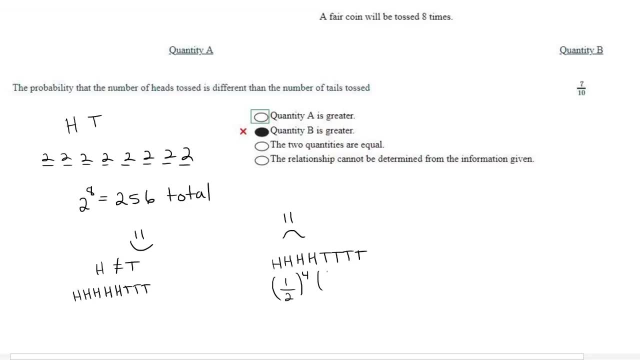 fourth. Okay, And if I get four tails in a row, that's going to be one half to the fourth, And that's going to equal one half to the eighth, just like before, And that's going to equal one over 256.. So this is just one case of the 256 right there. So the question is now: how many of these? 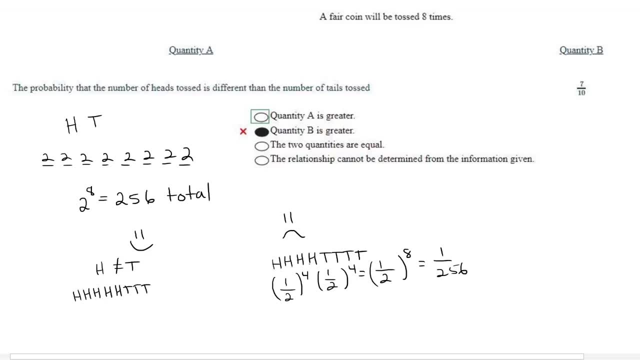 different cases do I have where I have four H's and four T's. Remember, these T's can be in the middle of the H's or the H's can be in the middle of the T's, right? So we're just going back to our good friend, you know. 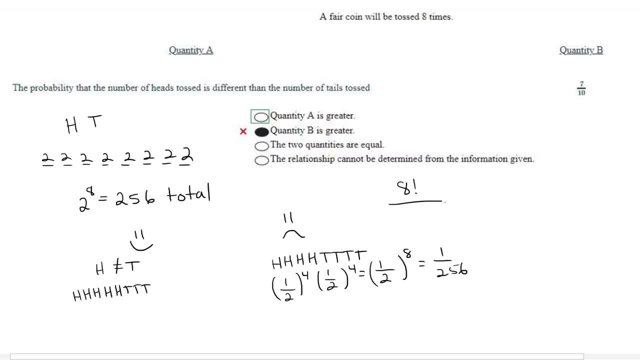 the total over the repeats. So the total is eight factorial. how many H's are there Four? How many T's are there Four? And so what do we get? we get eight times seven times six times five, over four times, three times, two times one, And we can do a lot of simplification here, right? So you know. 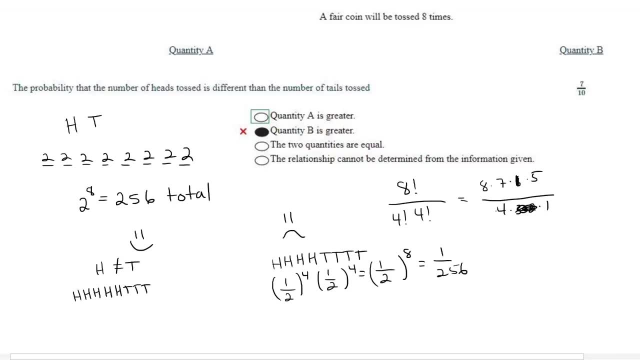 the three and the two. well, those go away, so does the six, that four goes away and that turns into a two. So what do we get? we get: 35 was at 70.. Alright, so we have 70 total possibilities. Now remember: 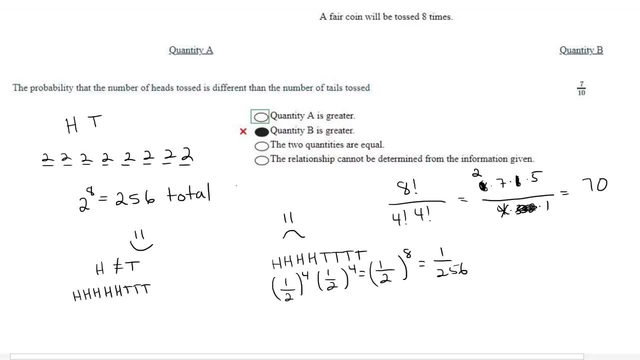 these possibilities make me unhappy, So I need to subtract them from 256: 256 minus 70. And what is that going to equal? that's going to equal what is it? 186? Is that right, Alright? so these number of these possibilities make me happy, because that means they're not. 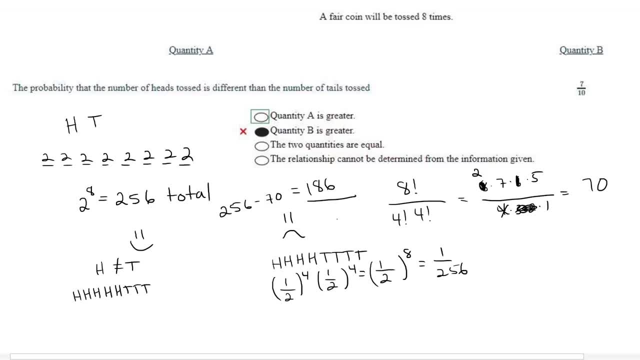 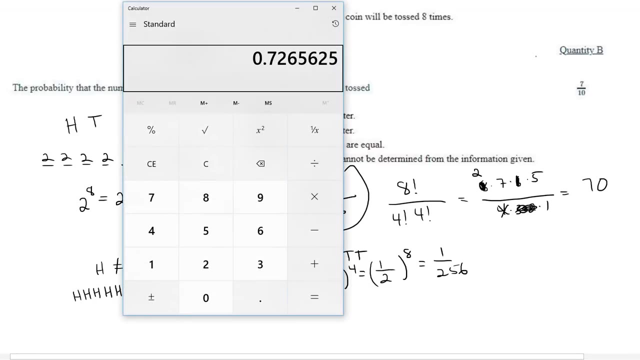 equal, because I subtracted all the things that make me unhappy. So 186 over the total number, which is going to be 256.. And then, finally, I'm going to compare this number to seven over 10, and see which one is bigger: 186 divided by 256.. So it looks like a is bigger, point seven. 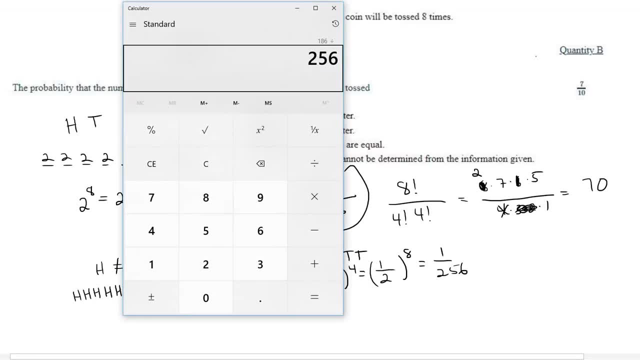 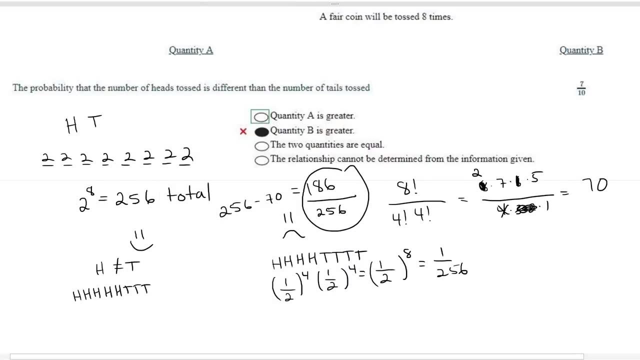 bigger One: 86 divided by two, 56.. So it looks like a is bigger, 0.72 is bigger than seven over 10.. So the correct answer is going to be a, as indicated by this green box right here. All right, So that was a pretty fun one. The principle again is: do the easier calculation. 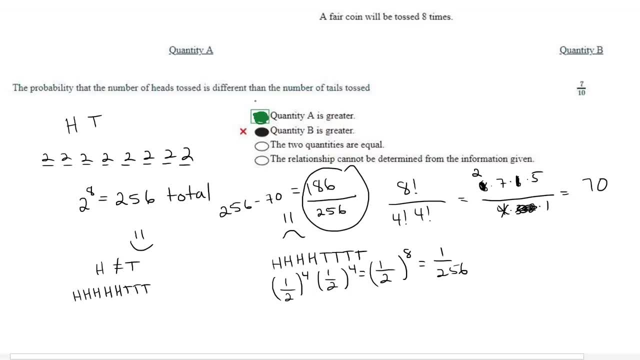 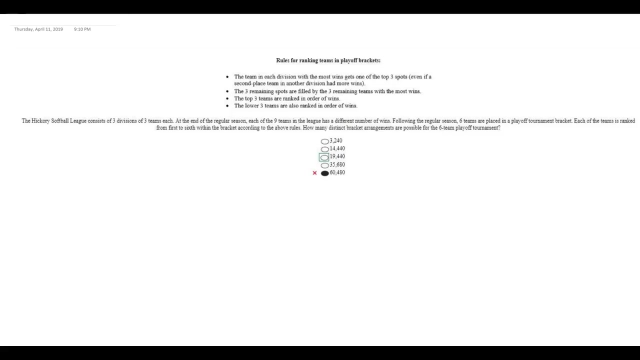 Sometimes it's easier to calculate What you want. Sometimes it's easier to calculate what you don't want and then take it away from the total. In the last two cases it was easier to take away what I don't want. So this is the last one that was requested, And at the top we have some rules for ranking teams. 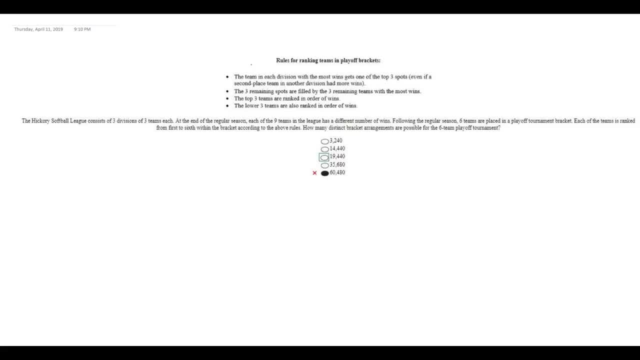 in the playoff brackets. And you know, the first rule says the team in each division is going to be the first team in each division. So the first team in each division is with the most wins gets one of the top three spots. Okay, The three remaining spots are filled. 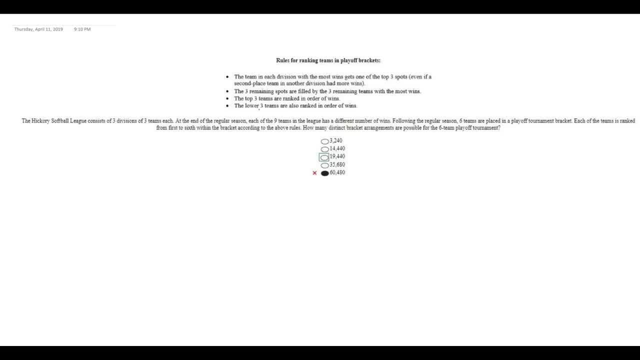 by the three remaining teams with the most wins. The top three teams are ranked in order of wins And the lower three teams are also ranked in order of wins. So it says this: Let's take a look. Okay, So the Hickory Softball League consists of three teams. 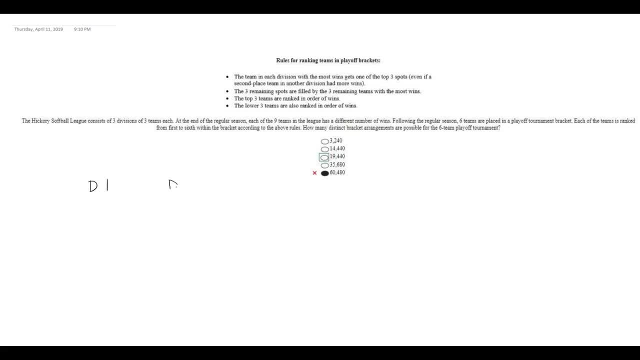 So three divisions. So we have D1, D2, and D3.. At the end of the regular season, each of the nine teams in the league has a different number of wins. a different number of wins. Okay. So we have nine teams, So three in each. So we got A, B, C, D, E, F and then G H. 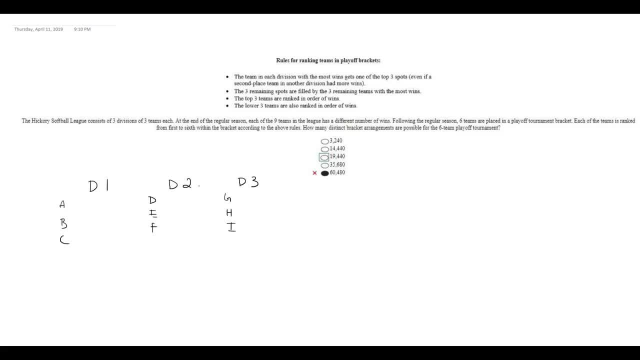 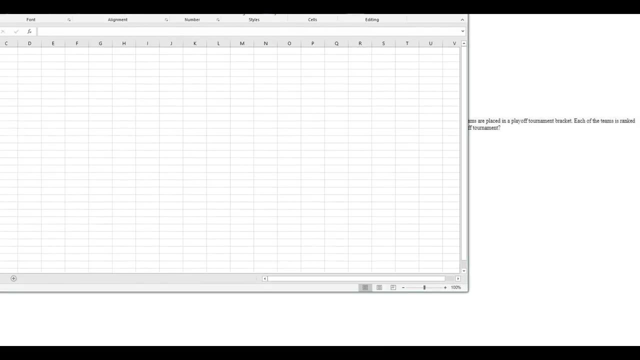 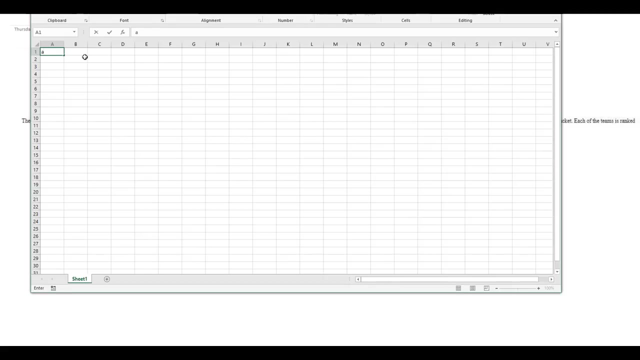 i, so they all have a different number of wins. okay, well, that's interesting. how about we get some excel action going so we can assign some different wins to people here? all right, there's excel, so we have nine teams, right, so we got a, b, c, d, e, f, g, h, i. 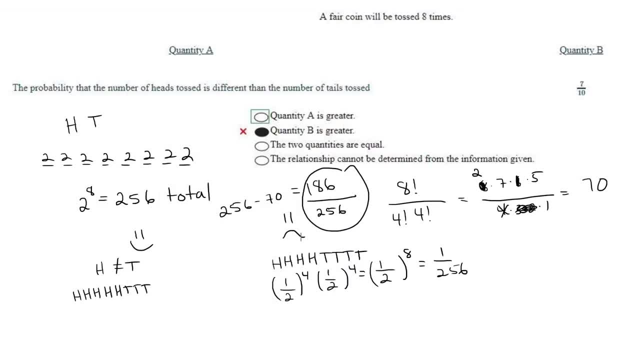 two is bigger than seven over 10.. So the correct answer is going to be a, as indicated by this green box right here. Alright, so that was a pretty fun one. The principle again is: do the easier calculation. Sometimes it's easier to calculate what you want. Sometimes it's easier to calculate what you don't. 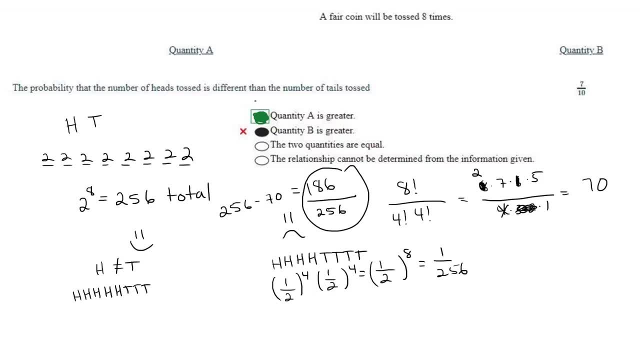 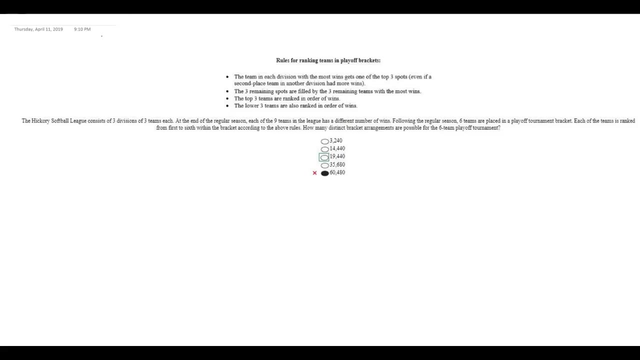 want and then take it away from the total. In the last two cases it was easier to take away what I don't want. So this is the last one that was requested. And at the top we have some rules for ranking teams in the playoff brackets And you know, the first rule says the team in each division with the most. 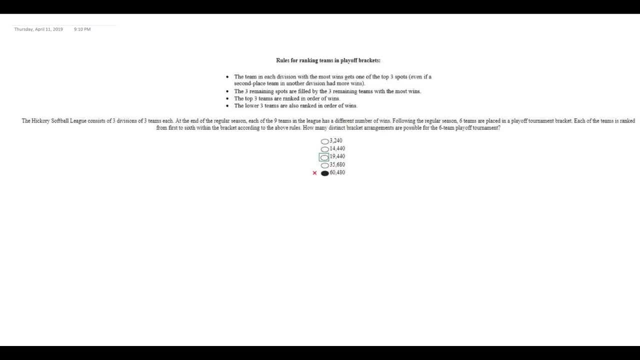 wins gets one of the top three spots. Okay, the three remaining spots are filled by the three remaining teams with the most wins. The top three teams are ranked in order of wins And the lower three teams are also ranked in order of wins. So it says this. Let's take a look to get to one of the 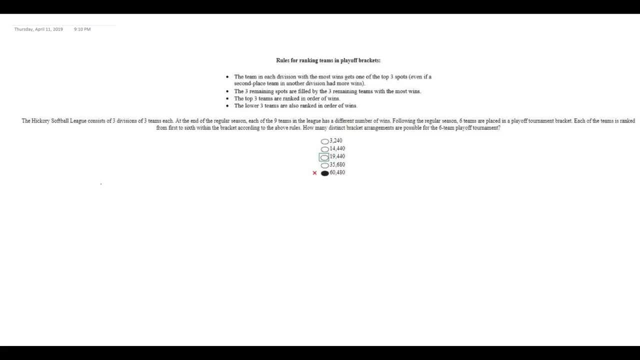 top three. Okay so the Hickory softball league consists of three divisions, So we have D1, D2, and D3.. At the end of the regular season, each of the nine teams in the league has a different number of wins. 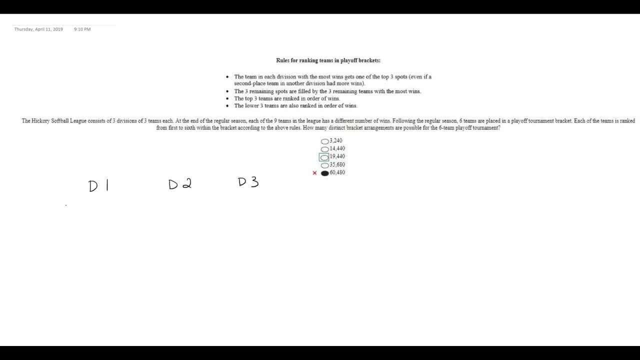 Okay, so we have nine teams, so three in each. So we got A, B, C, D, E, F and then G, H, I, So they all have a different number of wins. Okay, well, that's interesting. How about we get some Excel action? 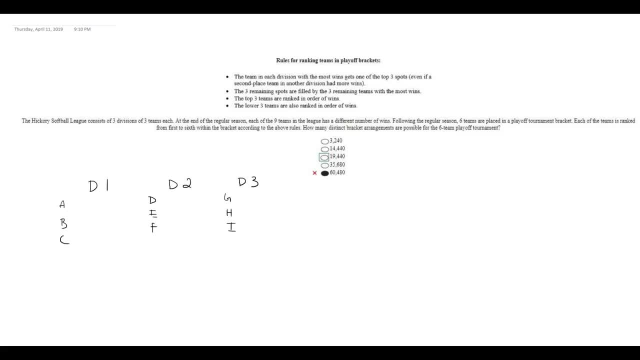 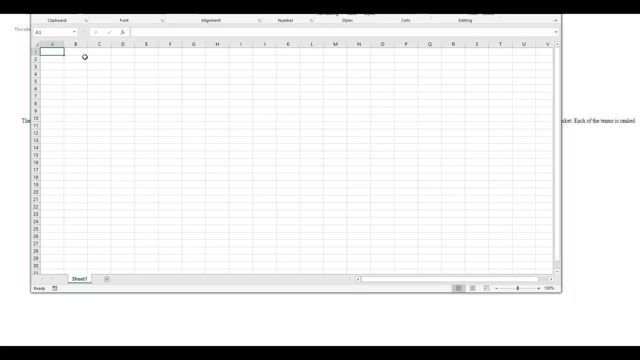 going, So we can assign some different wins to people here. All right, there's Excel, So we have nine teams right. So we got A, B, C, D, E, F, G, H, I, All right. 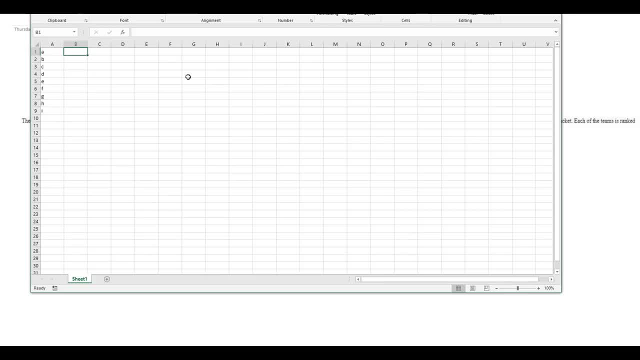 and let's just say: yeah, let's just keep it easy. Let's just talk about, let's say: 1, 2,, 3,, 4,, 5, 6,, 7,, 8,, 9.. And then let's: 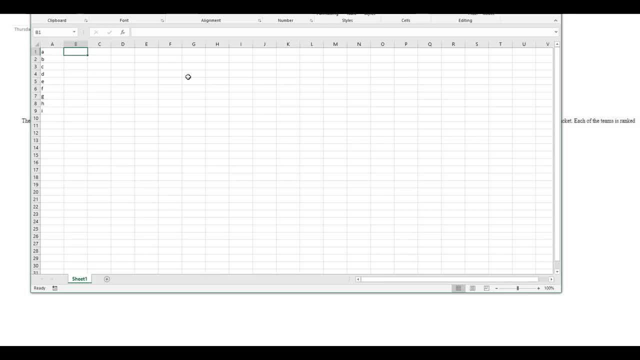 all right, and let's just say: um yeah, let's just keep it easy. let's just talk about: let's say one, two, three, four, five, six, seven, eight, nine, and then let's randomize this. all right, this will be kind of fun, okay. all right, let's take a look. 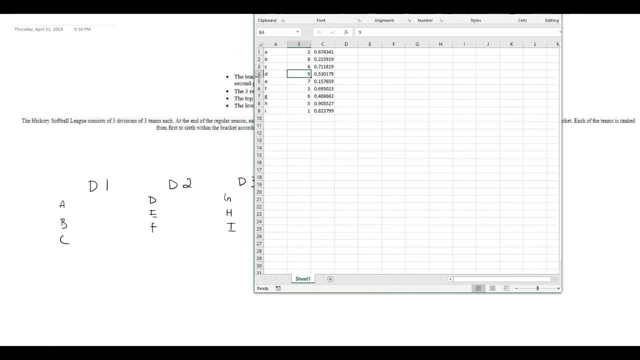 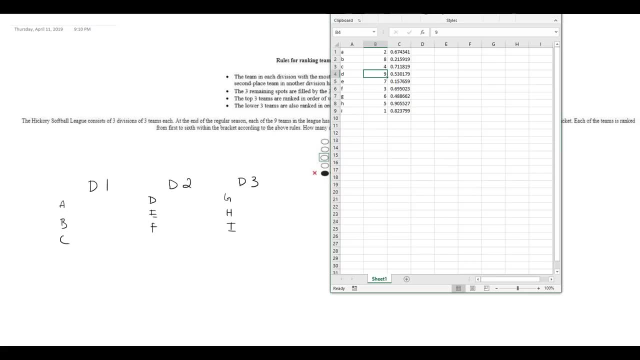 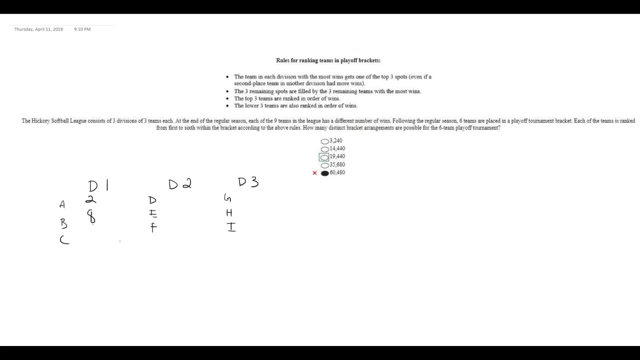 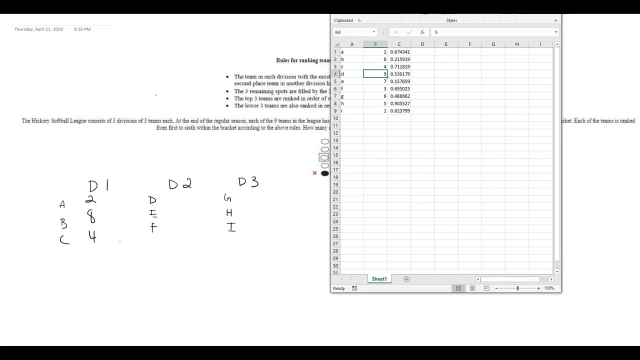 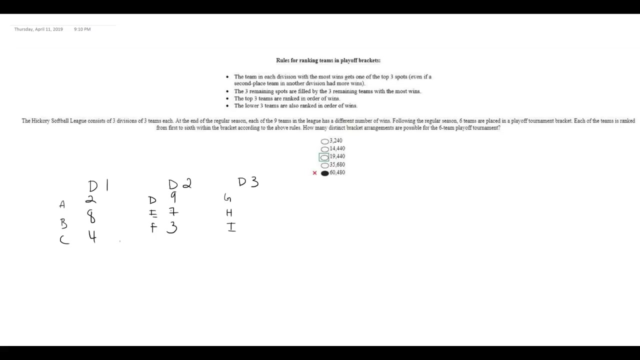 so let's write this down according to excel: a, b, c is two, eight, four. all right, two, eight, four. d, e, f is nine, seven, three, and then the last one, g, h, i is six, five, one. so according to these rules, the 16 playoff would look like this: 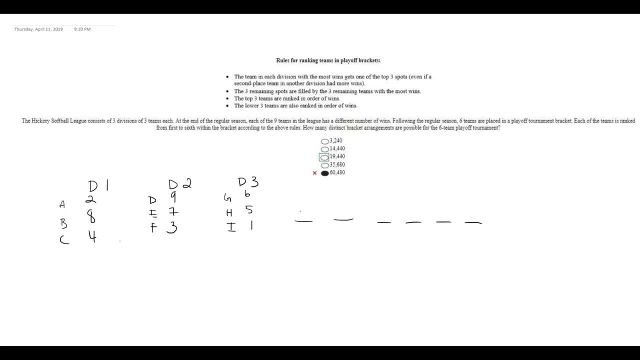 five, six. okay, the first one is the top division leader, which is d. okay, so that's one. number two would be the next division leader, which is b and then g. okay, the three remaining spots are filled by the three remaining teams with the most wins. all right, so how many wins did d have? 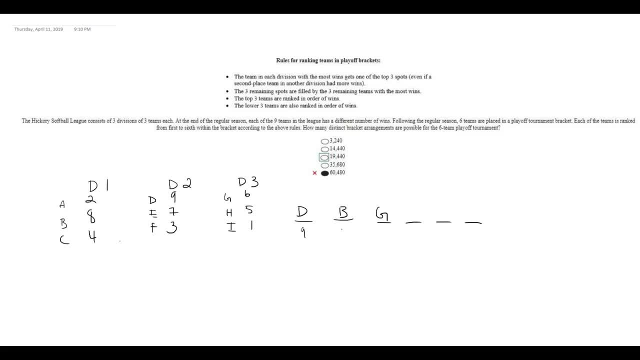 nine, how many? did b have eight, and then g had six. okay, so who had seven wins? that would be e. who had five, that would be h, and then, finally, who had four, that would be c. okay, all right, so that's one possibility right here. so that would be seven, five, four. so that's just one possibility. the question is asking me how many? randomize. Okay. so we have a team that's ranked in order of wins. So we have D1,, D2, and D3.. At the end of the regular season, each of the nine teams in the league has a different number of wins. So we got A, B, C, D, E, F, G, H, I, All right, and let's just say: yeah, let's just keep it easy, Let's just talk about, let's say, 1,, 2,, 3,, 4, 5, 6,, 7,, 8,, 9.. And then let's randomize. 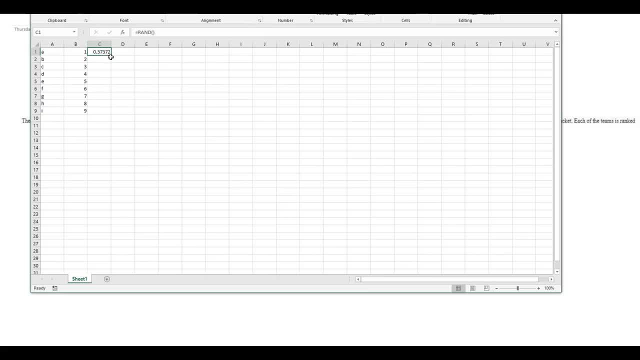 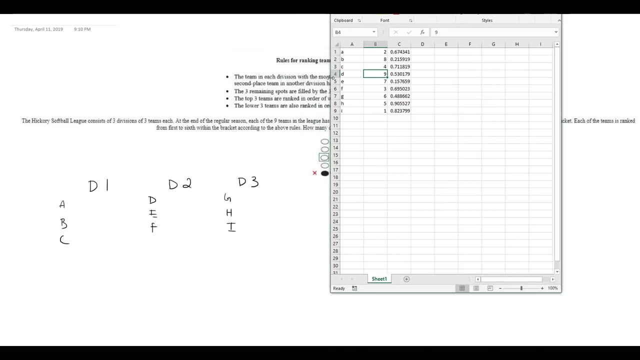 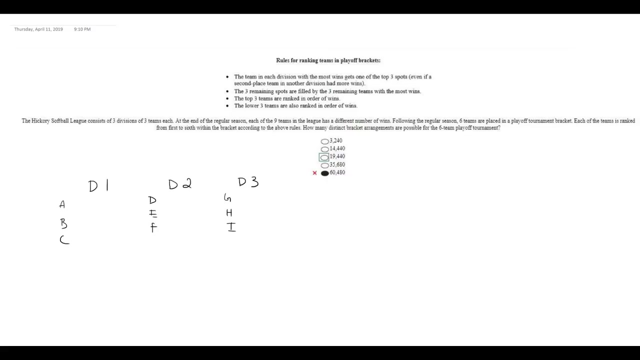 This. All right, this will be kind of fun, Okay, All right, let's take a look. So let's write this down. According to Excel, A, B, C is 2, 8, 4.. All right, 2, 8, 4.. 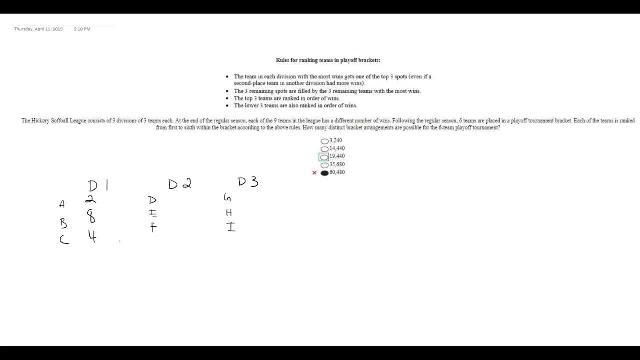 Alright, DEF is 973, and then the last one, GHI is 651.. So, according to these rules, the six-team playoff would look like this: five, six- okay. The first one is the top division leader, which is D. okay, so that's one. 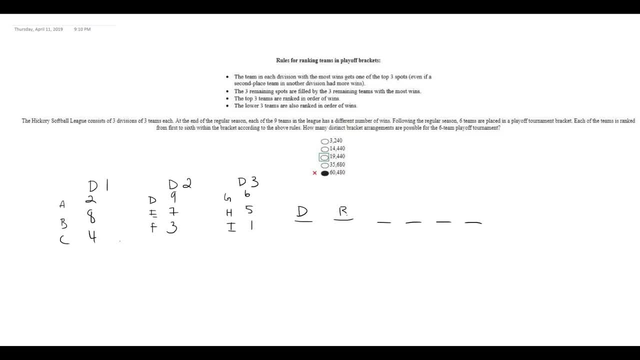 Number two would be the next division leader, which is B and then G. okay, The three remaining spots are filled by the three remaining teams with the most wins. All right, so how many wins did D have? Nine, How many did B have? 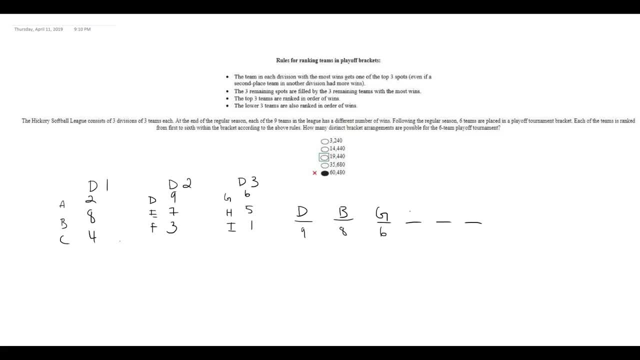 Eight, And then G had six. okay, So, who had seven wins, That would be E. Who had five, That would be H, And then, finally, who had four, That would be C. okay, All right. so that's one possibility, right here. 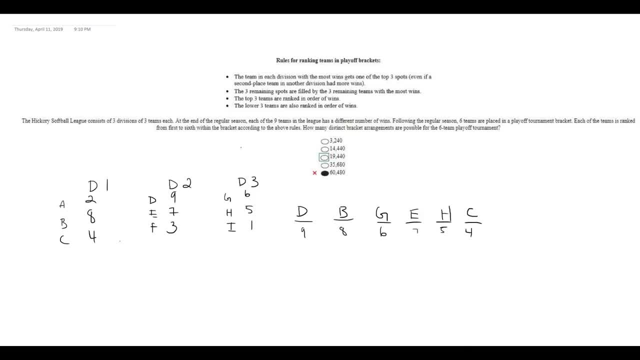 So that would be seven, five, four. So that's just one possibility. The question's asking me: how many different possibilities do we have? Do we have? okay, pretty interesting question. two, three, four, five, six, all right. 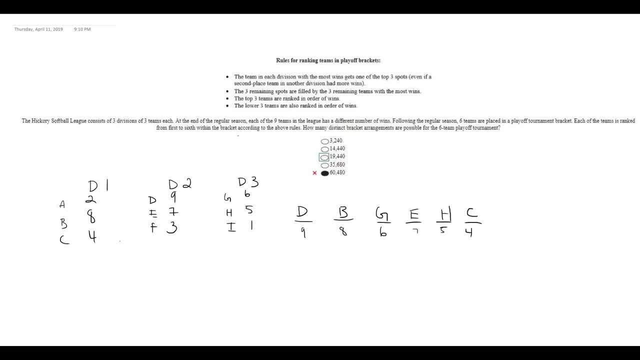 different possibilities do we have? do we have? okay? pretty interesting question. two, three, four, five, six, all right. so in this first spot, you know, let's clean the season. could be anybody right, could be anybody nine, nine choices, but you automatically lose two of them because you can't have the same division right here. so imagine it's f, okay. so 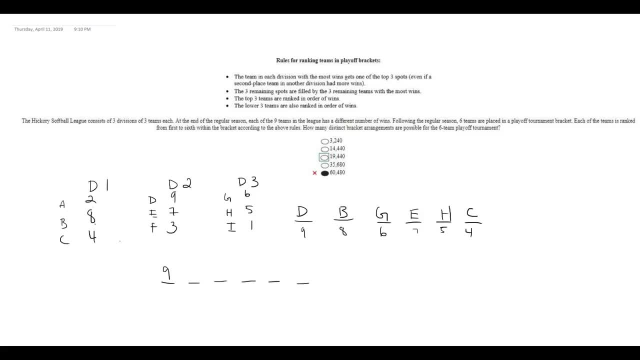 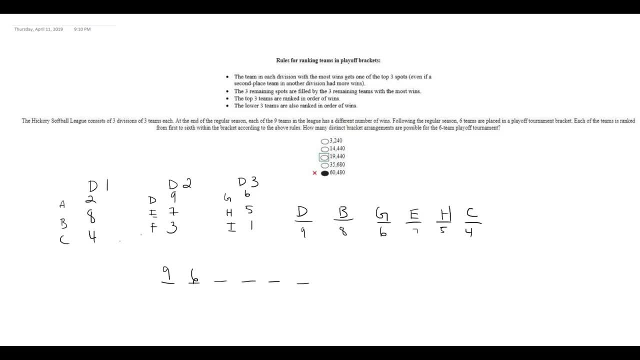 means i'm only going to have what is it? three choices, okay, so these. this is the the way it works. for the first three, all right, and then you're choosing the top three, anywhere, anywhere. so now it's just the number of choices you have left. so you have six. 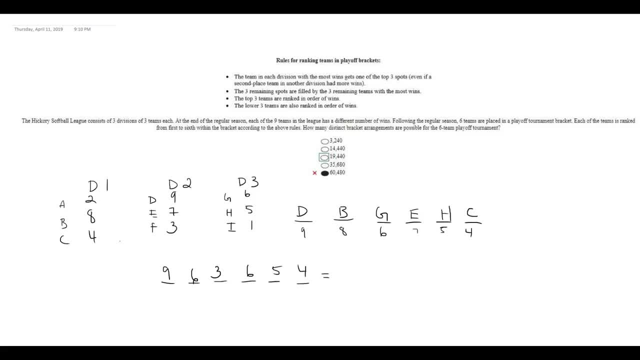 five four. i think that's the correct answer. so let's multiply all those together and see what we get. okay. nine times six times times three times six times five times four. nineteen four forty: that is the correct answer. times five times four. nineteen four forty: that is the correct answer. 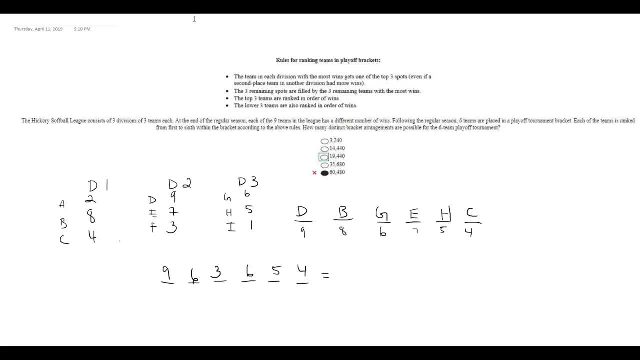 so obviously i went through this very slowly just because i was kind of curious how it worked. not really necessary, but interesting, but definitely interesting. so the correct answer is going to be c. now really, the the last three spots are pretty straightforward: 6, 5, 4. 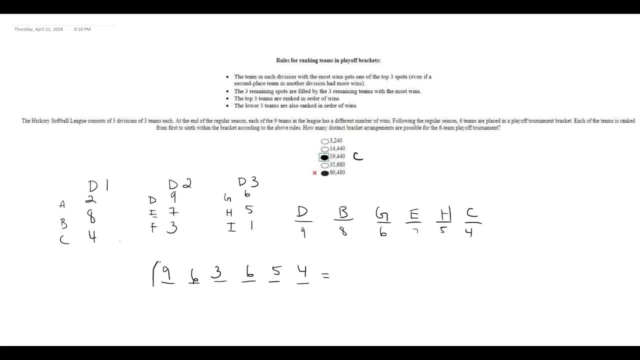 this is the part that you have to understand, that you need to do so. here we arebur dollar, economic B2. così, that's the tricky part, Because in the first case it could be anybody, But then, once it's anybody, you lose two of the spots. two of the spots, So the next one can only be six, and then you lose. 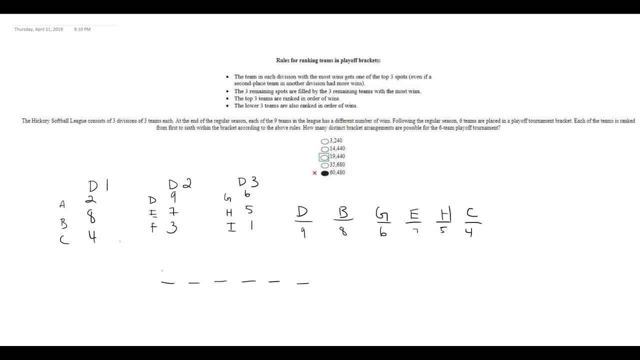 So in this first spot, you know, let's clean the season. Could be anybody right, Could be anybody nine, nine choices, All right, All right. So then again you have two choices. You automatically lose two of them because you can't have the same division right here. 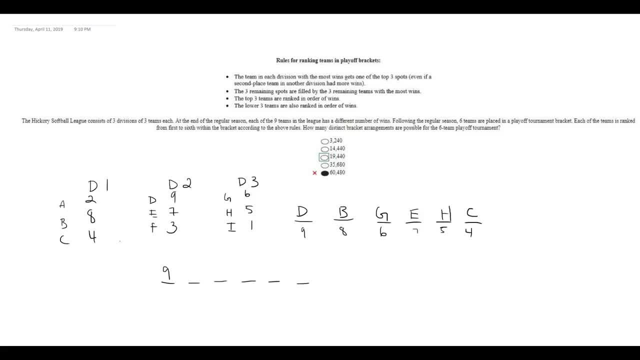 So imagine it's F, okay, So the next one can't be E or D, So I only have one, two, three. I have six choices right there, Okay. And then now imagine it's like I, for example. well, that means I lose two more right there. 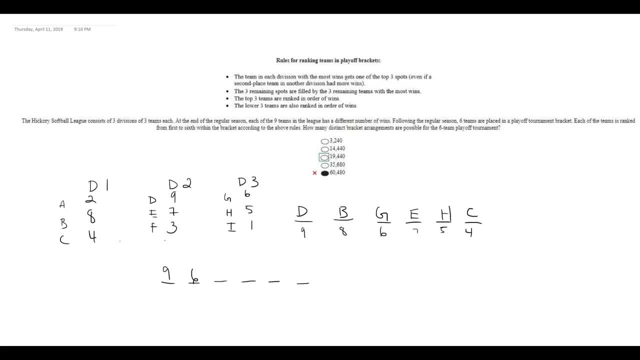 I lose two more, So that means I'm only going to have- Okay, was it? three choices. okay, so these. this is the the way it works. for the first three, all right, and then you're choosing the top three, anywhere, anywhere. so now it's just the number of choices. 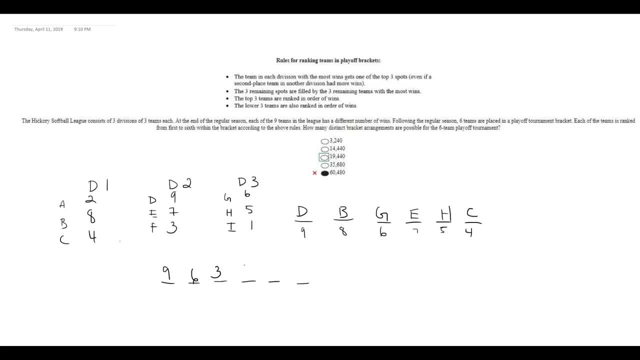 you have left, so you have six, five, four. I think that's the correct answer. so let's multiply all those together and see what we get. two, two, two, two, two. okay. nine times, six times, three times, six times, five times four. nineteen, four, forty: that is the correct answer. so obviously I wouldn't. 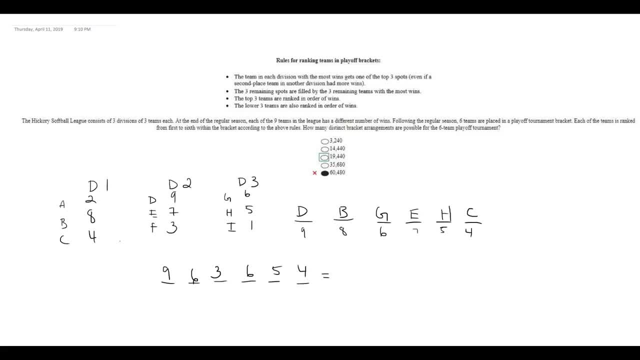 be going through this very slowly, just because I was kind of curious how it worked- not really necessary, but interesting, but definitely interesting. so the correct answer is going to be C. now really the. the last three spots are pretty straightforward: six, five, four. this is the part that you have to understand. that's the tricky part, because in the first case it could be anybody. 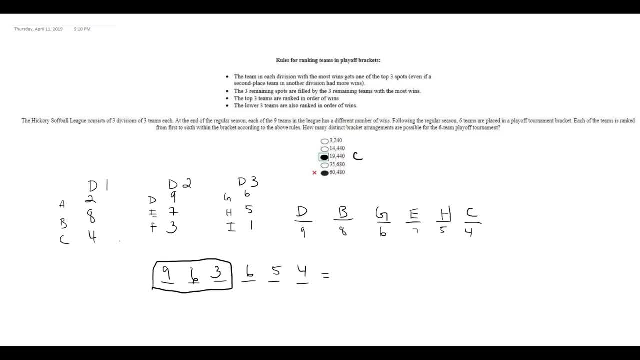 but then, once it's anybody, you lose two of the spots. two of the spots, so the next one can only be six, and then you lose two more and then it can only be three. all right, so that was fun. thank you, guy or girl on Reddit. I hope you found this helpful.